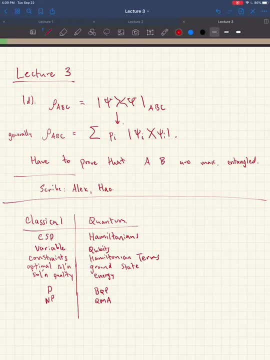 to BQP and QMA, which we'll talk about in depth today, And last time we talked about the Cooke-Levin theorem. So there's a Cooke-Levin SAT formula and this corresponds to a construction known as the Feynman-Kataev Hamiltonian Okay, which 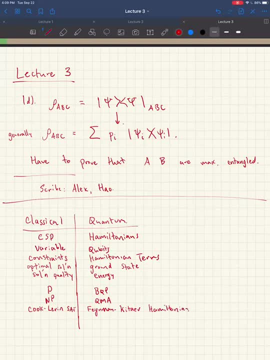 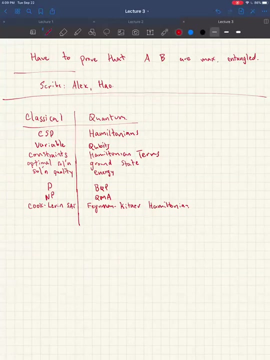 we hopefully will get to today. All right, So this is the dictionary. Let's keep this in mind. Last time we saw a definition of what local Hamiltonians are right, So we talked about K local Hamiltonians. This notion comes from physics. It's a way to describe physical systems and the local interactions between. 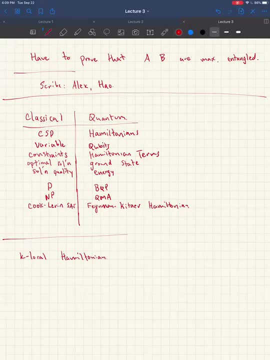 particles in these systems. But you know, the way we want to view it in this class is as a quantum analog of a constraint satisfaction problem. So it's a Hamiltonian acting on NQ. NQ bits is a two to the N by two to the N permission matrix. That is a sum of local. 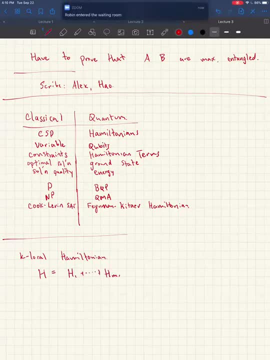 terms right Where these local terms are, the constraints on our qubits, And last time we saw. you know why. it's the generalization of constraint satisfaction problems. For example, we can write the max cut problem, which is a classical optimization or classical constraint. 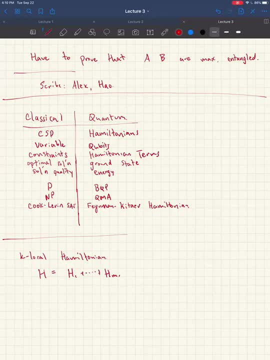 satisfaction problem as a Hamiltonian. Okay, Right, So the classical max cut. you know, if you have a graph then the corresponding Hamiltonian would be. you know, for every edge in the graph you have this Hamiltonian term, which is the Pauling's, that matrices acting on qubits U and V And the ground states. 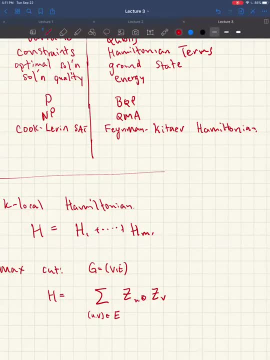 of this Hamiltonian will be. you know that the ground space is spanned by optimal solutions to the max. cut problem right And in the lecture notes from last week you can take a look. There's a derivation explaining why the ground states of this Hamiltonian are the, these classical strings that tell. 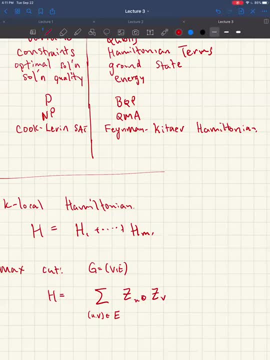 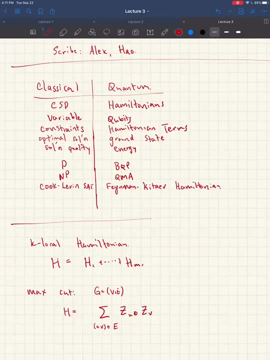 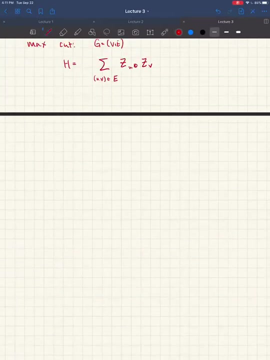 you how to obtain a max cut in this particular graph. But the max cut problem is a classical problem, right? So what are some other examples of local Hamiltonians that are more genuinely quantum, that exhibit true quantum behavior? So I'll just write down a very well studied and well-known family of Hamiltonians known. 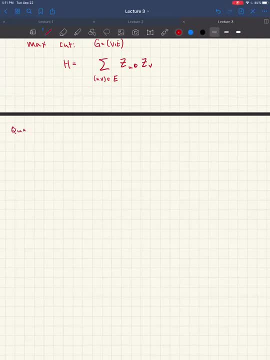 as the Heisenberg model. Okay, So this is actually not a single Hamiltonian, but it's a family of Hamiltonians that's parameterized by some parameters. So it's a Hamiltonian That's a function of four real numbers. We'll call it J, X, J, Y. 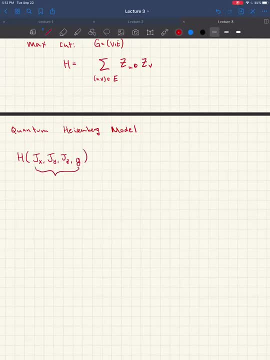 J, Z and G. These are all real numbers, These are real parameters And you know, this is some Hamiltonian that acts on n, g And it's really close to a real, real number, So it's qubits. we can think of these qubits as, say, living on a line or in a grid or at 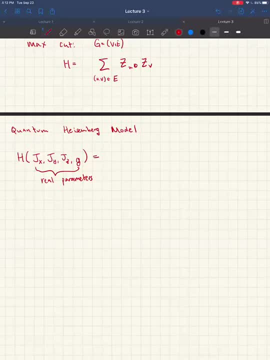 some lattice or maybe some more general graph. For now we'll just think of it. as you know, the qubits are arranged in a line, So the Hamiltonian terms are grouped into different buckets. We have one bucket that corresponds to the, the poly x-terms. so on qubits i and its neighbor i plus 1, we have these this term xi. 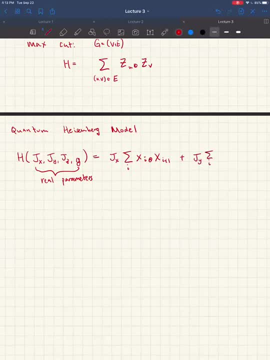 tensor xi plus 1.. We also have a similar thing with the poly y matrices, the z matrices and we also have this term that runs. we have single qubit x terms. So for every combination of real numbers, jx, jy, jz and g, we have a different. 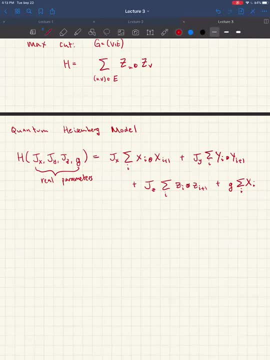 Hamiltonian and each of these Hamiltonians has a ground energy, has a ground state, has a whole spectrum right And the properties of these ground states can vary wildly depending on what parameters you choose for these j's and g. So, for example, you know this actually recovers the original max cut. 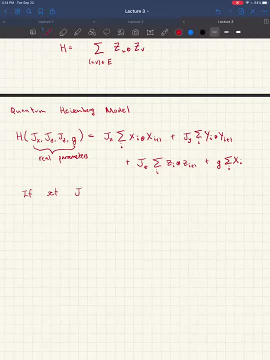 like if you set, you know, j, z equals to 1, g equals to 0, and jx equals, jy equals to 0. This is just the max cut, the classical max cut problem. An interesting choice of parameters, though, are when you set jx, jy, jz, all to be the same, Let's 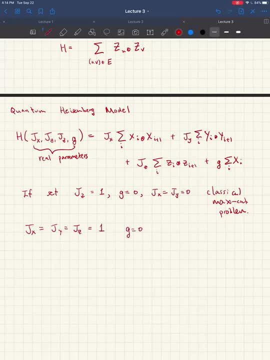 say we set them to 1 and maybe we'll just set them to 1, and maybe we'll set them to 1 and maybe we'll just set g equals to 0. And this is known sometimes this is called the quantum max cut problem. And this is a very interesting model because 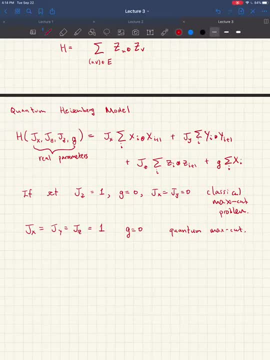 the ground states are in general, very quantum, like they're highly entangled. They have lots of quantum entanglement going on, And one way to see why this is kind of like a genuinely quantum describes like a quantum system. well, if you look at these terms, they don't necessarily. 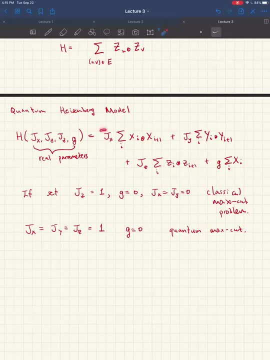 commute with each other, Right, Because you know so. all of these j's are equal to 1.. So you have these. you know this balance of x, y and z terms And each of these constraints are kind of asking the qubits to do. 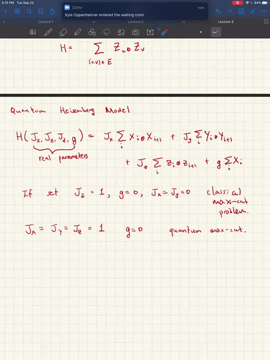 something you know, different in different bases, And the ground state is trying to satisfy all of these hamiltonian terms best as possible, In fact. so you know, let's sort of zoom in on just a specific i. So we have, let's say, the i-th qubit and the i plus first qubit, And on these 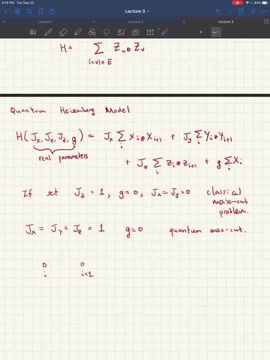 two qubits. we have xi and xi plus one, asking these two qubits to be in a certain state, You know. similarly for yi and zi and zi plus one. Does anyone know what the ground state? let's say? you know, we just have this Hamiltonian on. 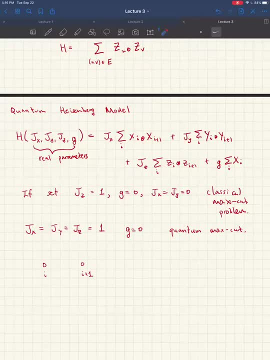 two qubits. Does anyone know what the ground state of this Hamiltonian would be? Any guesses? So this is a two qubit Hamiltonian. Would it not be something like spread equally among all the eigenstates, now like of each of those operators? 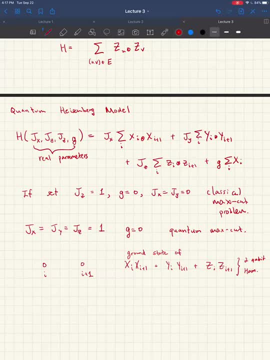 Well, let's see. So this, if you sum all these terms up, it will have a unique ground state. This: it will be true that the ground state of this, the sum of these things, will be- I think yeah, will be- the ground state of of each of these individually. This is not always true, by the way. 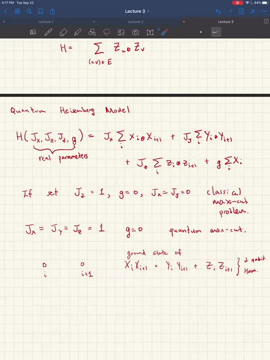 But in this particular case you do have this property, So this shouldn't. this is not too hard to calculate, Like you can run it through MATLAB or something or you know- take five minutes to write it out. But if you do the computation and you diagonalize this four by four matrix. 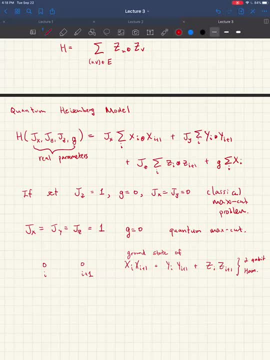 you'll get that the, the ground state of this matrix will be an entangled state. It's this thing called the singlet. So this looks kind of like the maximally entangled like an EPR pair that we've seen before, Except, you know, the two bits are flipped. 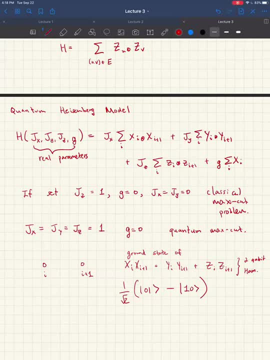 They're, you know, anti-aligned and there's like a minus sign between, but it's basically the same as a, as a maximally entangled state, And it's kind of interesting because between every consecutive pair of qubits, i and i plus one in order to like try to satisfy each of these terms. 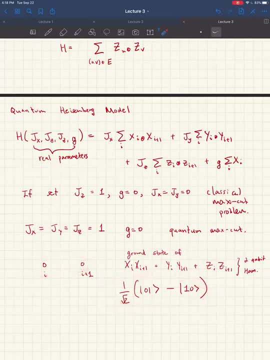 these two qubits really want to be in this maximally entangled state. But actually, as you know, you're you're working on in the problem set, it's not possible for, let's say, one qubit to be maximally entangled with its right neighbor. 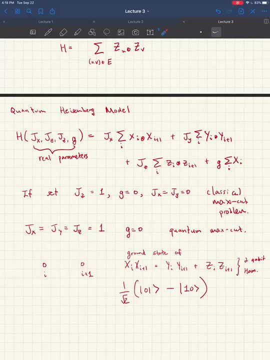 And also maximally entangled with its left neighbor. So what happens is when you sum up many of these terms together in this quantum max cut Hamiltonian, you have a bunch of constraints that are not all simultaneously satisfiable, because you're asking the qubits to do. 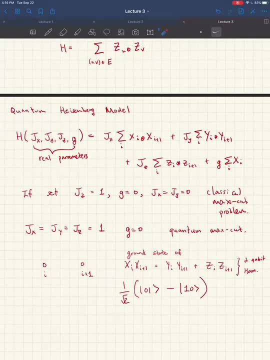 things that are not possible. So what happens is the the ground state just tries to, you know, satisfy some of them and sacrifice satisfying the other ones, And there's like lots of really interesting structure that that comes up. So and I actually, you know, I'm not an expert in this area- 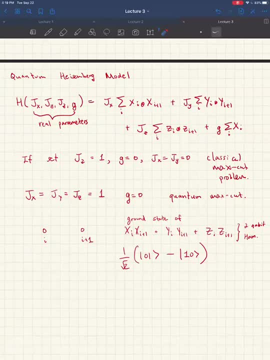 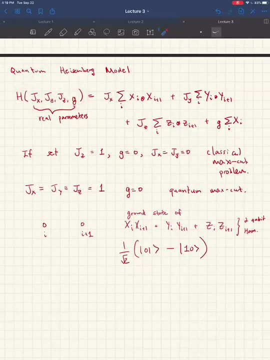 but as far as I can tell, I don't know if there's any exact description of what the ground state of of this model is. I mean, people sort of study this model to death and they have like lots of really good understanding, but I don't. 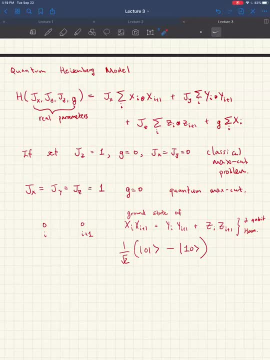 know if anyone can sort of write down like a closed form expression of what the ground state is. But I mean, if you know about this I'd be happy to. I don't know for sure, but it might be the case that for one dimension you can. 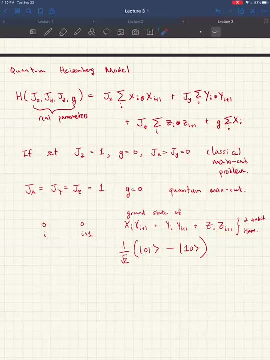 solve it exactly. but as soon as you get into two dimensions, then you get some frustration and then you cannot solve it exactly. I know this is the case for the Hubbard model. In one dimension you have an analytic formula for it, but as soon as you increase the 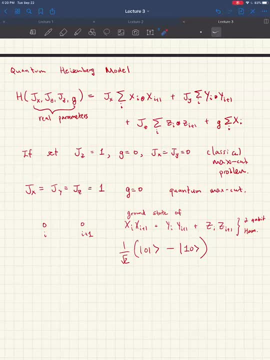 dimensionality. it's hard to solve, Right, right, Although I think even in this and for this specific model in in one dimensions, like if all the qubits are in, like in a ring, we it's still frustrated like you cannot, you know, from this monogamy entanglement. 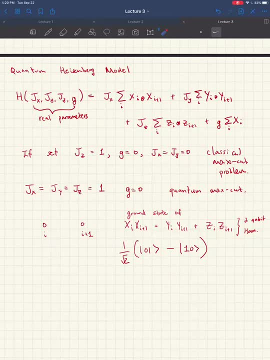 you cannot satisfy all of the the constraints simultaneously. Oh, I see Adrian seems to have a link to a solution. Okay, But yes, you know this, analyzing these sort of Hamiltonians is like the bread and butter of lots of what people do in physics, from what I 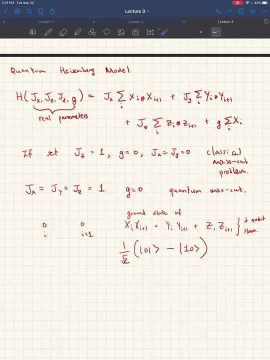 understand And there's like a huge literature around it and there's lots of interesting things going on. So in this class we're not going to focus on solving any particular Hamiltonian. I mean, that's something for like a condensed matter theory course. 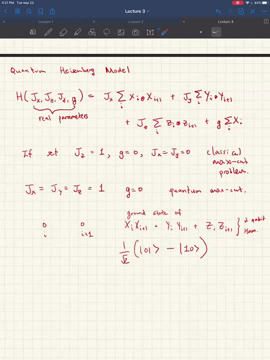 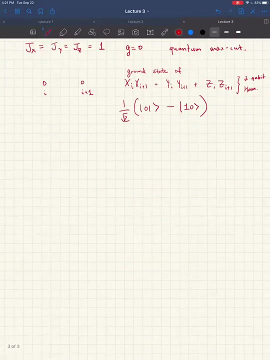 But instead we're going to take a step back and think about this problem of solving local Hamiltonians more abstractly, like just solving Hamiltonians in the abstract Right. so I want to phrase this as a computational problem, like a problem that you would want to solve on a computer and not just pen and paper. 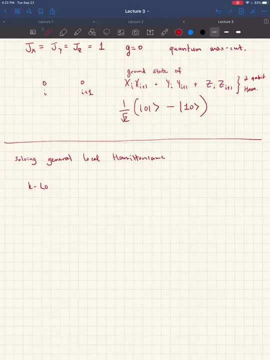 So I'm going to define the k-local Hamiltonian problem. I'll just abbreviate as k-local ham. I'll give two subscripts: a and b. These are numbers. so k, a and b are numbers. So this is going to be a decision problem. 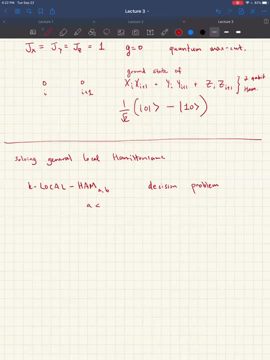 Okay, And a and b are real numbers. k is an integer that represents the locality, like how many qubits each of your Hamiltonian terms act on And the instances of this problem, like you know, the input to the computer when. 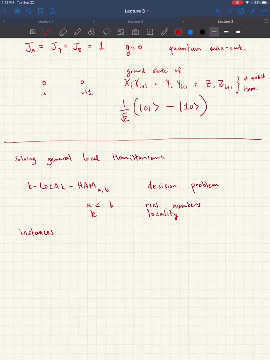 you're trying to have the computer solve it is going to be some k-local Hamiltonian acting on, So you get a bunch of A's and B's on n qubits. okay, So each of these are k local terms. So like the description to the computer would be how many qubits are acting on n. 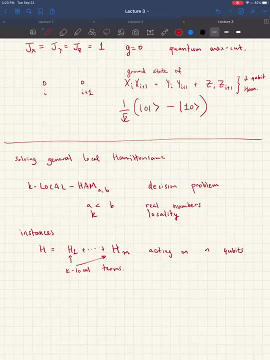 How many terms are there? m, which subset of k qubits the term H is going to act on, and then you have to specify what the term is. So, since it acts on k qubits, you just need to specify a k qubit operator. so a 2 to the k by 2 to the k matrix. 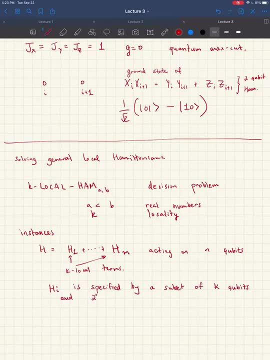 And then, once you've written down all this data, this tells you everything you need to know. Well, it tells you what the Hamiltonian is. So these are what the instances are. and then what is the decision problem? You have to have a yes. 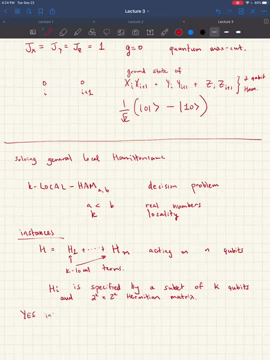 and no instance. So the yes instance is when the ground rate. yeah, I didn't get, I didn't quite get what the a and B parameters were and why a smaller than B. oh, I'm gonna say what it is right now. okay, yeah, yeah, no, perfect. so so the essence is to say that the the ground 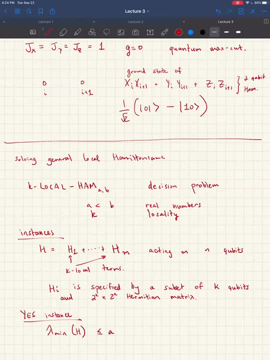 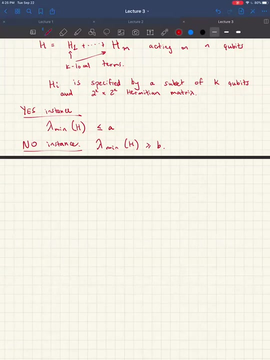 energy of this local Hamiltonian, the minimum eigenvalue is less than this number a, and the no instance is when this minimum energy is is greater than B, or at least B. I don't know if you, I don't know, is that off screen or something. maybe let me do this so you present this local Hamiltonian to the 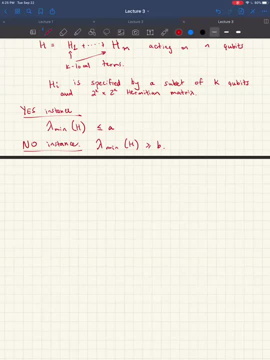 computer and you're asking the computer: tell me, is it a yes instance or is it a no instance? is the ground energy less than a or at least B, and your computer has to do something to to try to figure this out if your Hamiltonian doesn't. 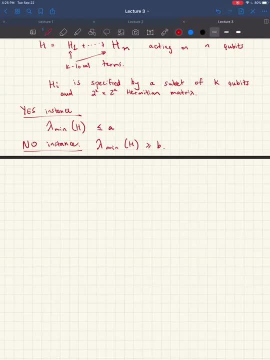 satisfy either one of it. maybe the minimum energy is somewhere in between a and B. we don't care like. we just think that's sort of like not part of the discussion. you're promised that the input to the problem satisfies. it's either yes instance or a no instance. so that's what this 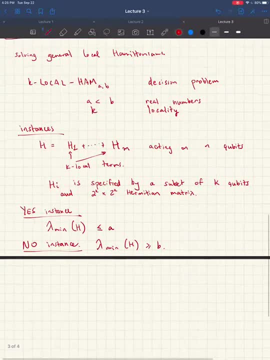 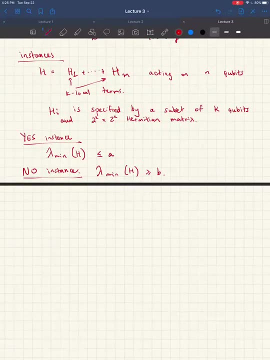 decision problem is: this is what this K local ham a, B you have to do: figure out the minimum energy, yeah, like so we don't care about the values of a and B, we just pick two a, two values- a and B- and we proposed this. okay, if it's smaller than. 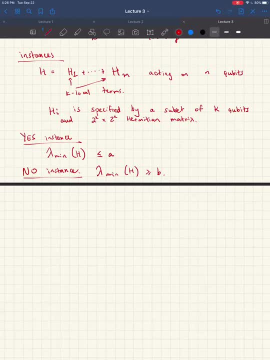 a, it satisfies the instance yes instance, and if it's greater than B then it satisfies the the no instance. that's it right? are there any constraint on choosing a and B? so right now there a and B can be anything. you, yeah, you tell the computer what a and B you're interested in. but then you fix it and then it has to try. 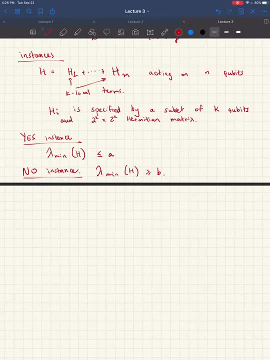 to solve it for that. a and B, okay. okay, but later we'll add more constraints on what a and B are. for example. just to jump ahead, a and B can't be like infinitely close together, because then you're asking: I mean, that's like two, fine, a distinct, distinguishing problem. right, you have to have a little bit of. 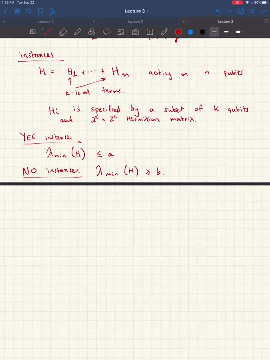 gap to, to allow the computer some room to distinguish between the two. okay, just so I can wrap my head around what that means. do you have like a concrete example of some decision problem and for which what a and B would be? okay? that's a great question. so so here's an example. let's let's go back to the classical. 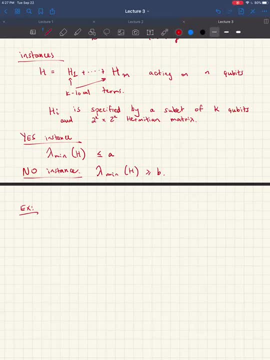 case, just at least for me, it's very helpful to ground my intuition and what what this means. so, so I claim that this max cut problem, you know, you walk up with this graph and then we had this Hamiltonian that I wrote before. so you have this Hamiltonian which is the sum over Z U, tensor Z V. so it turns out. 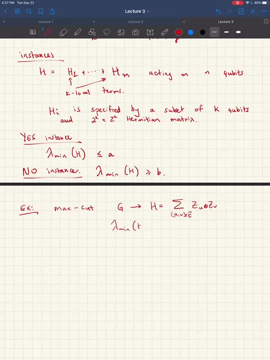 that the the minimum energy of this, of this Hamiltonian. it's going to be the number of edges of your graph minus I think it's twice the size of the maximum cut. okay, so the lecture notes from last week will derives this. so you see, can take a look, but just take my. 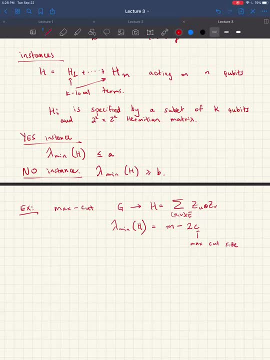 word on this for now. so you know that abstractly. but of course you're interested in finding out what the max cut is like. someone hands you a graph like: what is the max cut? this can be phrased as an instance of this K local ham problem. so max cut is it's sort of a to local Hamiltonian. 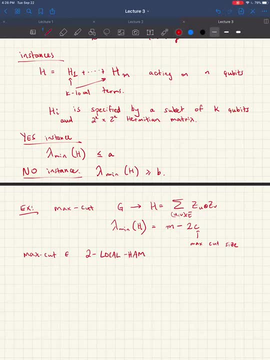 problem, because these are, these are two local terms. and what are the a and B? well, the A could be. let's say, you're trying to determine whether, basically, you set two thresholds, like you want to know, is the cut bigger than 2C1 or is it? 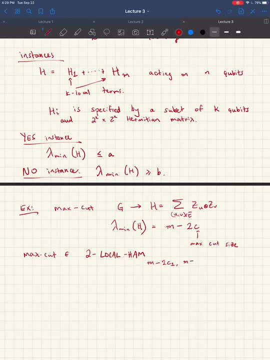 smaller than 2C2.. Okay, so C1 and C2 are different cut sizes, like how many edges you can cut. So if you could distinguish between whether the minimum energy is below this amount or above this amount, that equivalently tells you whether the max cut is. sorry, I think I messed this up. this is C2 less than C1. 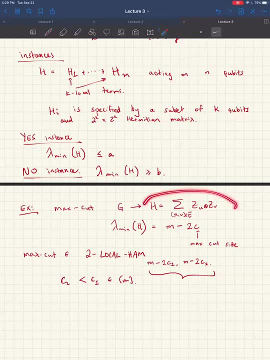 The point is, suppose you you took this Hamiltonian. you took this Hamiltonian and you knew that its minimum energy was less than M minus 2C1. that tells you that the max cut must be at least as large as C1.. On the other hand, if the minimum energy is greater than M minus 2C2, 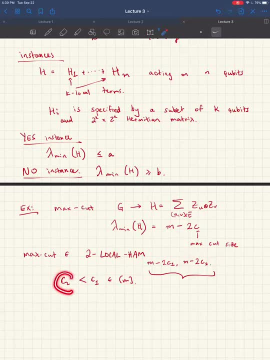 the max cut has to be smaller than C2.. So this gives you a way of it's like another way of calculating the max cut size, at least between two different cases. Okay, so like it's basically trying to like fit these two values so that your 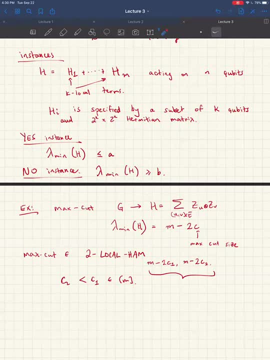 solution basically makes sense, right. So you have this kind of a gap or a range where you know if, if that is the case, if it is below that, it's a yes problem. but you don't care how or like what the actual range is right. Of course you say: 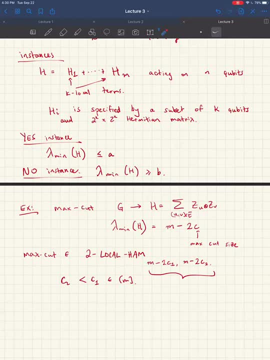 well, what if I want to know more information, like, what if I want to know what the actual minimum energy is or what the actual max cut size is? Well, you can do. you can sort of sweep the A and B until you've homed in. you know, you can. 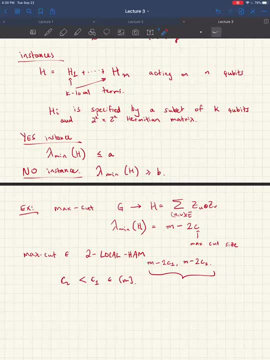 do like a binary search. is it less than or bigger than this? Okay, yes, then let me shift the A and B until you've homed in on the right value. Okay, so the reason we put this A and B is just to put it in in the in the language of a decision problem. 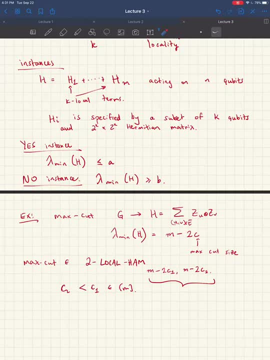 Yeah, good questions. Any other, any other questions? We need to make sure that we understand this. What happens if it falls between the gap, like between A and B There? then we sort of there's, we don't care. yeah, then we sort of kind of give up. 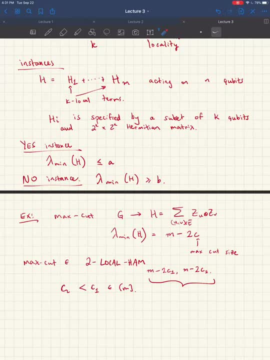 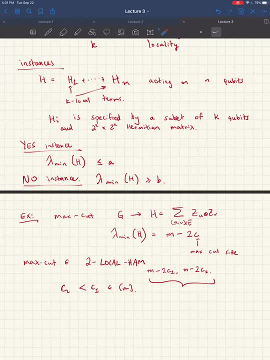 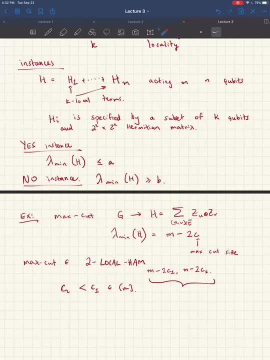 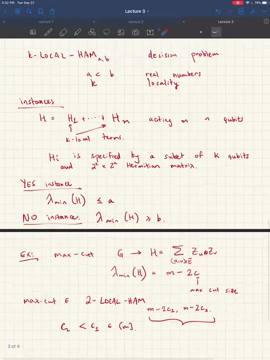 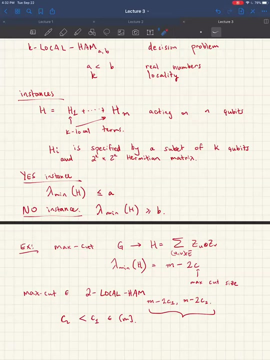 here or can, A will be A cannot equal B, because then they like the yes and no instances should be disjoint. Okay, So this decision problem, this K local Hamiltonian it's- it's going to be like the, it's sort of like the, the most important, like decision problem that we'll consider in the same way. 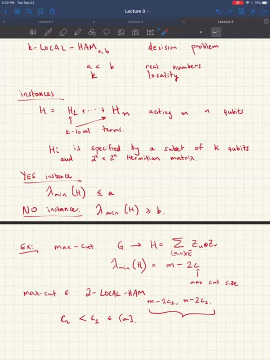 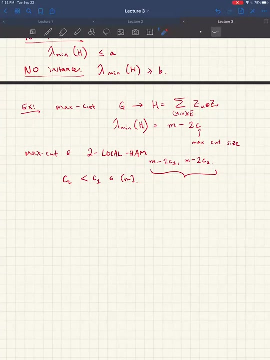 that, for example, KSAT or 3SAT is important to the theory of NP completeness. right, This is our analog, our quantum analog of KSAT. All right, So what is the? you know, I've defined a decision problem. We can then ask: what is its complexity? right, Like, just like. 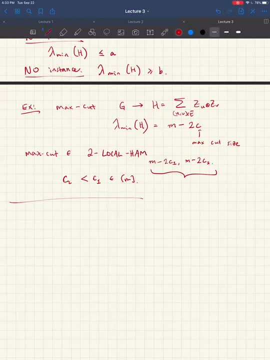 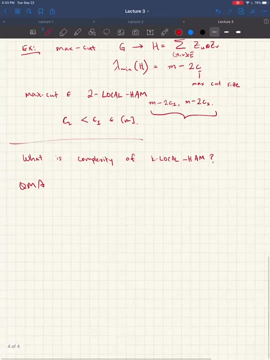 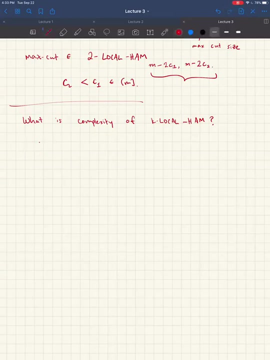 classical CSPs have NP completeness. like: is there an analog for quantum CSPs? And this brings us to the notion of QMA and QMA completeness. Okay, So now we start talking about complexity. Actually, before I go there, let's let's just start with the quantum analog of P, which 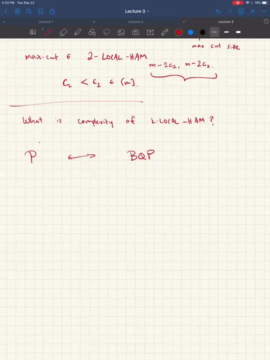 is this thing called BQP? What does this stand for? This stands for bounded error, quantum polynomial time. Okay, Okay, And remember that complexity classes. they're sets of decision problems And this is a set of decision problems that can be decided or solved by polynomial time, quantum algorithms. 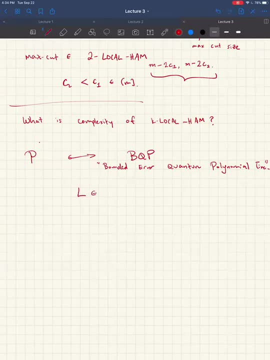 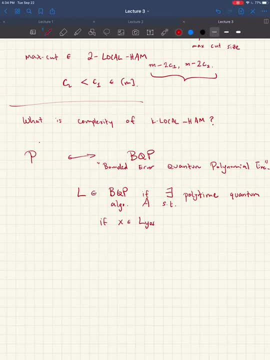 a yes Instance of whatever decision problem you're thinking about, then when you plug in X into your quantum algorithm, it's going to output one with probability at least two thirds. And the reason we're talking about probabilities is because quantum algorithms are inherently probabilistic. 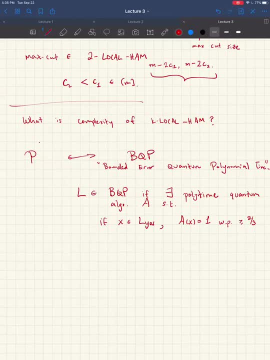 they don't always work all the time, we just insist that they work most of the time. And here we're picking two-thirds, just as some. it's kind of an arbitrary threshold. If x is a no instance, then x equals one with probability less than one-thirds. 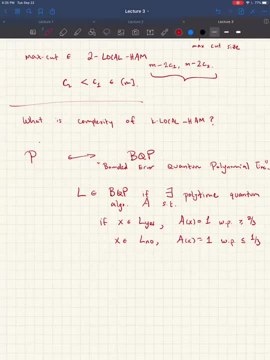 You can pick any two separated constants, like 99 for the yes case and 0.01 for the no case, and it just reflects how much confidence you have in the output of the algorithm. By convention we just like to choose two-thirds and one-thirds, but really it's arbitrary. 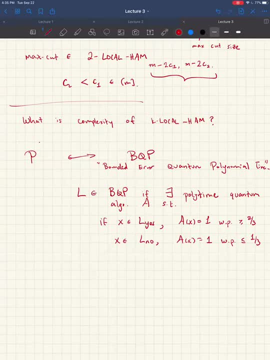 So what do I mean by a quantum algorithm? So there is something called a quantum Turing machine, but like its definition is that it's a quantum Turing machine. So it's a quantum Turing machine, but like its definition is incredibly unwieldy and like no one uses it. I mean, basically it was only defined in like the 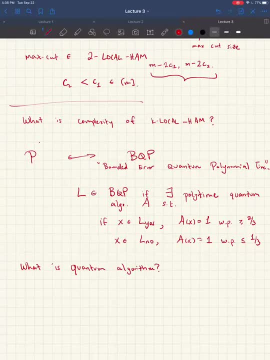 90s, when people started thinking about this. but then people quickly switched over to talking about quantum circuits because it's like much easier to think about. So by quantum algorithm what we really mean is that A is not just one thing, but it's an infinite family of quantum circuits. 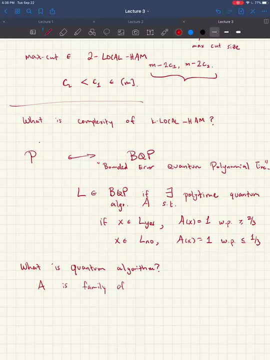 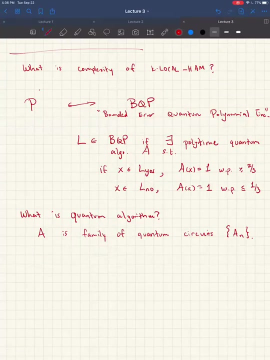 It's a quantum Turing machine. but it's not just one thing. but it's a quantum Turing machine, Okay, and it's indexed by this number, n, and it's going to represent the size of your input. So, for every input size, whether you're talking about an input size of, say, 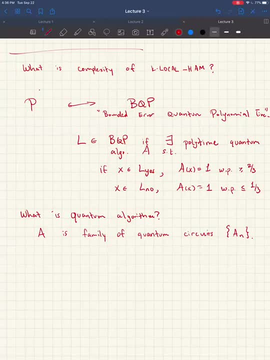 you know 100 bits or 200 bits or 2000 bits. there's a different circuit to deal with that For each input size. So if you walk up with some instance x that's n bits long, then A of x really means you know you have some quantum circuit. 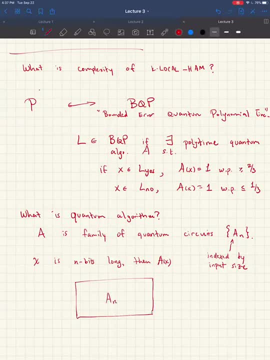 A, sub n, and in some portion of the circuit you're going to plug in as input the input you care about, and then in the other parts of the input you're going to put in zeros. This is like your ancilla qubits, They're like the scratch. this is like the workspace that your algorithm has to do. 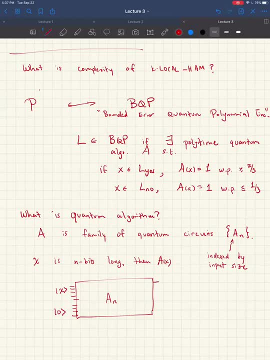 with computations, It runs its computations and at the very end you're going to have a single output, qubit, that you're going to measure to get the determine whether the answer is one or zero. And this is the output of A, of x. 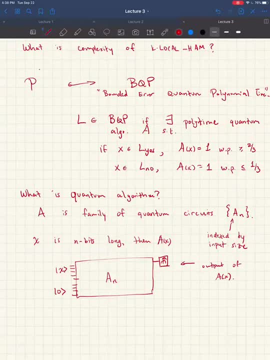 Okay, so that's what I mean by a quantum algorithm. We really mean this infinite family of circuits that depend on the input size. There's this additional constraint that these quantum circuits all have to be related to each other, like you can't have a totally. 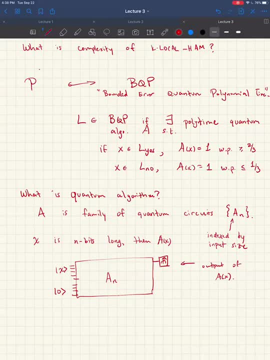 wildly different algorithm for every possible input size. So we also insist that this family is what's called uniformly generated. But you know. if you don't know what that means, don't worry so much about it. I mean, it basically means that there's a separate algorithm. that you know. 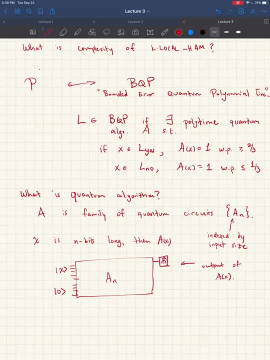 you tell it. I want the nth circuit of this family, and this algorithm will write it out for you. Okay, so let's see. let's see what this is. let's see what this is. let's see what this is. 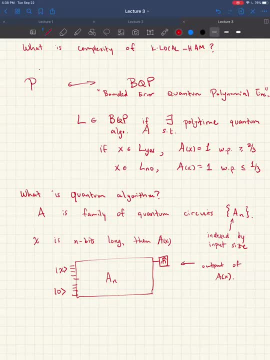 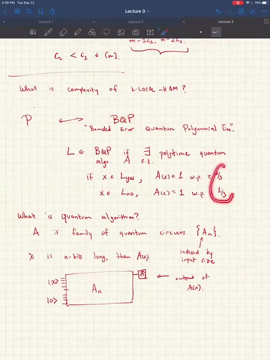 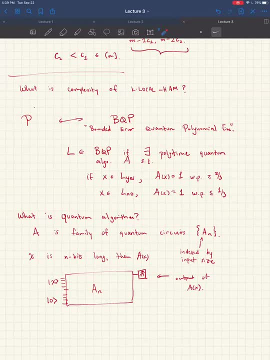 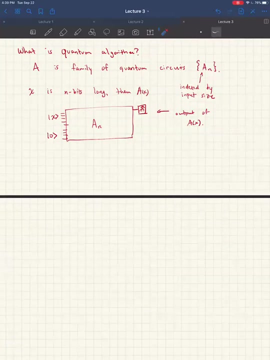 from each other. Like you know, the difference between your algorithm outputting one on a yes instance and outputting zero is significant, And this is, you know, roughly what we call significant. What's the implication of choosing these numbers? Would things be drastically different? 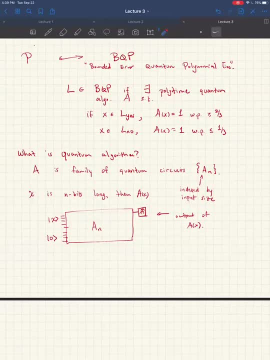 if we chose a different threshold to begin with. Good, it's not sensitive to what numbers you choose, as long as they're separated by a constant. So you could choose 99% or 1%, or, you know, 51% or 49%. 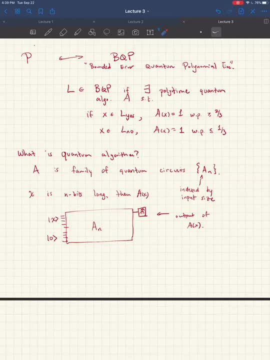 The set of problems that you can solve in polynomial time don't change because you can always amplify. Like if you wanted to get more confident in the answer of your algorithm, you would just repeat the algorithm as many times as needed, As long as it's not an exponential amount of time. 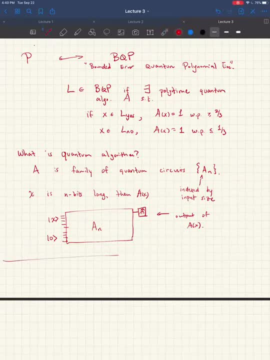 Exactly. So, just to now that you ask, the only requirement is that the. so this number is called the completeness, It's just a term, And this is called the soundness, And the only requirement is that the completeness minus the soundness is at least one. 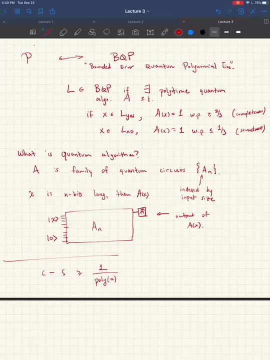 over some polynomial number in the size of your input. As long as this is the case, then you can always. if you wanted to boost up your confidence, you could always just repeat the algorithm a polynomial number of times. Okay, so that's BQP. 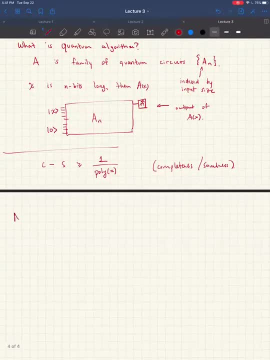 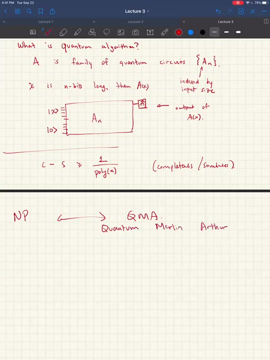 That's the analog of classical polynomial time. Now let's move on to NP, and it's analog QMA. Okay, so QMA stands for quantum. Merlin, Arthur, Hey, Henry, Yeah, Sorry, just a quick question about the nature of the circuits. 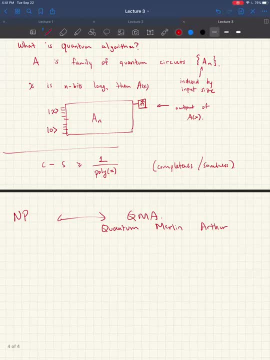 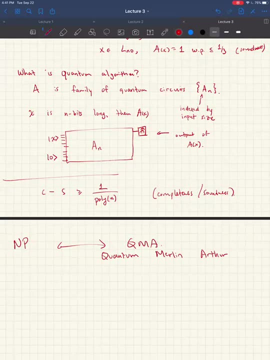 So what is the precise source of randomness? Is it just randomness that's inherent in the input qubits, Or is it also allowed to use some external sources of randomness? The randomness comes from measurement, So Sure, yeah, There's no, I mean everything. 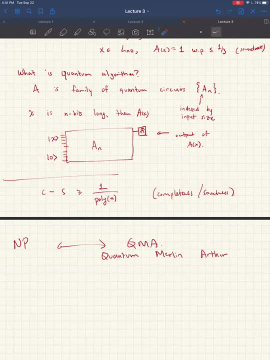 the input here is deterministic, It's just the input in all zeros. but the quantum algorithms can easily manufacture their own randomness, For example preparing the plus state and then measuring. in the standard basis You're gonna get zero or one, with probability half, for example. 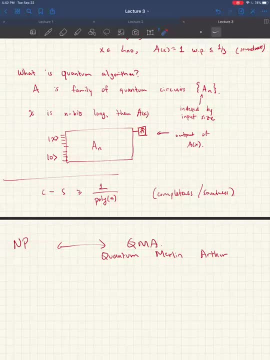 Sure right, sure Yeah. but generally speaking, most quantum algorithms we work with, whether it's like Grover's search or the Shor's algorithm, they're all probabilistic. They only output the right answer with two thirds probability, or something like that. 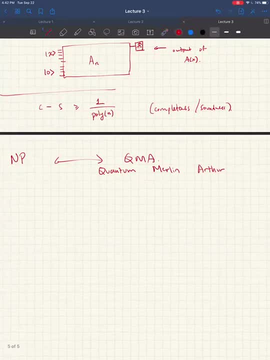 Yeah. so Alex was asking what is bounded error going to play? Yeah, that's just two thirds versus one third. Basically, as long as C minus S is at least one over polynomial, then that counts as bounded error. If it's one over exponential. 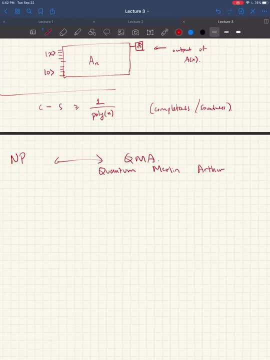 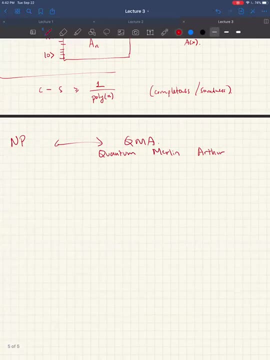 then that doesn't count as bounded error. That's a more powerful class actually. If you take the, so QMA, so this one should. you might be able to already guess what the definition of this should look like, But let's write it out. 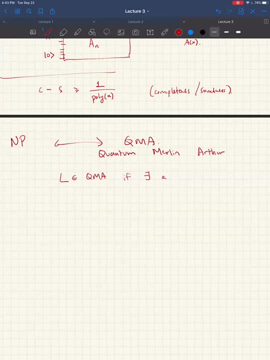 So a decision problem is in QMA If there exists a quantum polynomial time algorithm, a family of circuits, And this algorithm will take in two inputs, not just x, the instance, but also an additional input called the proof. So if you have a yes instance, there exists some quantum state psi such that 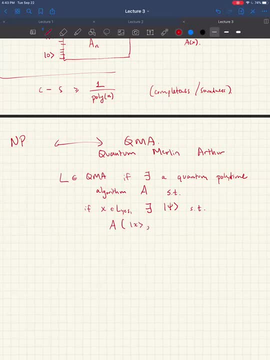 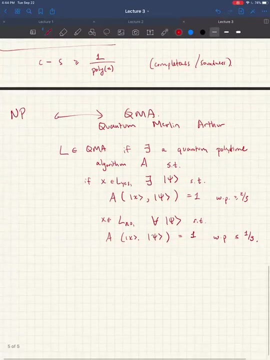 if you plug in your input and also this quantum state this accepts with this equals one with probability two-thirds And if x is a no instance, no matter what proof state you plug in, your algorithm is going to output zero or sorry, output one with probability at most one-thirds, And this state is called. 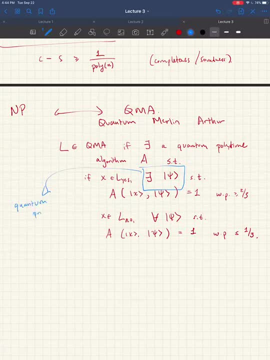 a quantum proof And you know this should ring a bell because this looks very much like the definition of NP, except the proof doesn't have to be just some string, it can be any quantum state. And just to draw out the diagram, like you know, we have a quantum circuit If x is n. 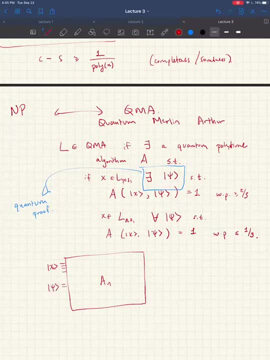 bits. then you plug in x here And someone- in this case you know, we like to think of it as Merlin- some all-powerful, all-knowing wizard, is going to hand this verifier, who we call Arthur, some quantum state psi. 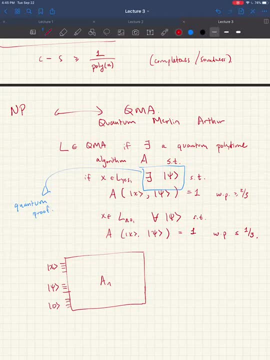 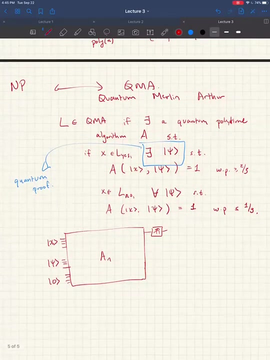 And Arthur is going to. and also, Arthur sets, you know, these ancilla qubits to zero and performs some polynomial-time quantum computation to determine whether x is a yes instance or no instance. Yeah, so where does this like terminology Merlin-Arthur come from? Well, it's based. 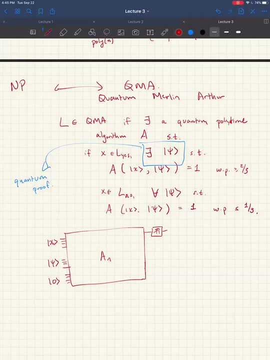 off of this like medieval folklore? Yeah, So where does this like terminology Merlin-Arthur come from? Well, it's based off of this like medieval folklore about King Arthur. you know the Knights of the Round Table And you know King Arthur. 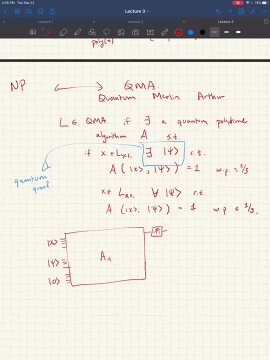 has this advisor who's Merlin. But Arthur doesn't necessarily always trust Merlin. So whatever advice Arthur gets from Merlin, he has to verify it, And that's where this you know so Arthur is. you know he's limited in his abilities, but he has to just verify. 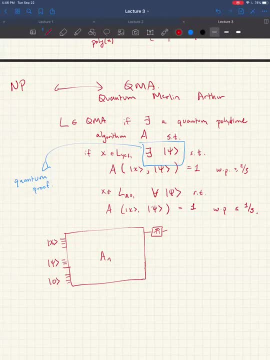 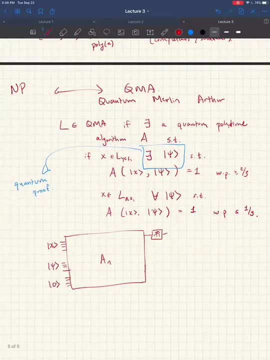 what Merlin tells him. Okay, Okay, Um. do we know who came up with these with his name? Oh, uh, yeah, I think, um the there's this um, computer scientist slash mathematician, Lassie Babai. he's at UChicago, he, he came up with these names back in the 80s. 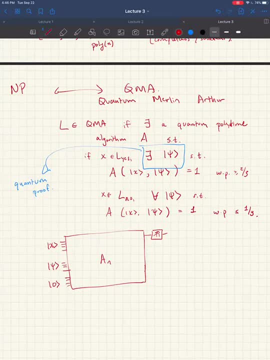 This was before quantum computing was really studied, and so, in classical complexity theory, uh, you know, people were just having fun coming up with these complexity classes and they defined a notion of Merlin-Arthur. um, uh, Merlin-Arthur proof systems, right? so it's exactly. 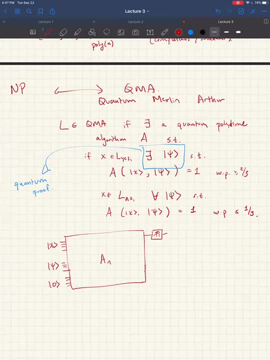 the setup like someone wants to determine, solve a problem. they can't solve it on their own, so they want to get a proof, just like in the NP setting um, and, and so we just like to think of them as characters. like Merlin tries to convince you of x is a yes instance, he gives you a proof. 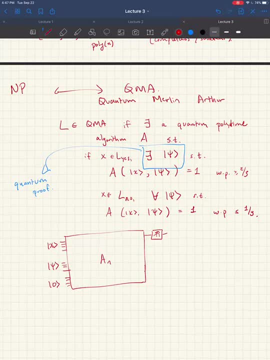 Arthur is able to perform polynomial time computations. Arthur is also able to do probabilistic uh computations, uh to determine, uh, whether that's the case. and so when quantum computing came around, they sort of just adopted this uh, this naming, Um. okay, so you know. so first let's uh one perspective on this definition of this complexity class, I mean. 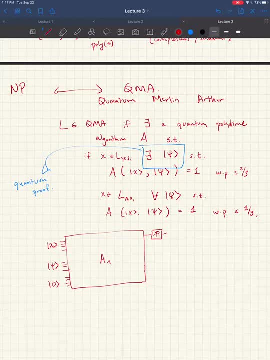 it seems like what? okay, well, it's kind of this abstract definition and, uh, what's interesting about it? uh, one thing that's interesting: is it really, um, uh, defines kind of this really interesting notion of a mathematical proof and kind of, uh, generalizes it. so the traditional notion of a mathematical proof? 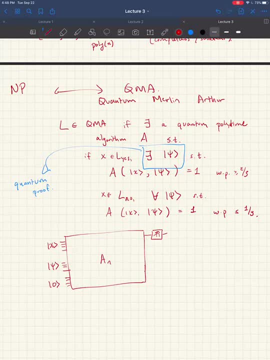 is that? well, someone says: here's a formal statement, x, which may or may not be true. um, maybe x is something like there's infinitely many primes, or p is, uh, not equal to NP, right, um? and to convince you of that x is true, someone will give you a mathematical proof. they'll give 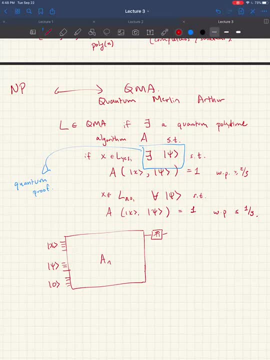 you like some table of text, okay, uh, and they hand it to you and you get this text and you sort of check line by line. okay, is it a valid deduction? uh, using, you know, the standard mathematical axioms, and at the end of this verification, you, you should walk away convinced. 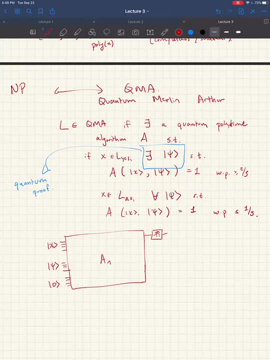 of whether x is true or not. right here we're saying: uh, why does the proof have to be some table of text, right? uh, some classical string? why not just have it be some arbitrary quantum state, which could be some weird entangled superposition between a bunch of particles? um, and to verify, 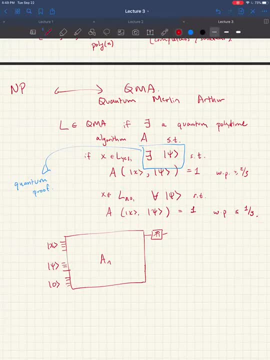 this quantum proof. you just perform some measurement on it, right, uh? or? or you know, maybe you can do something like run the quantum for your transform on these entangled particles and then do some measurement and at the end the measurement will tell you whether this is a valid proof or not, right? so it's kind of a funny, funny thing. 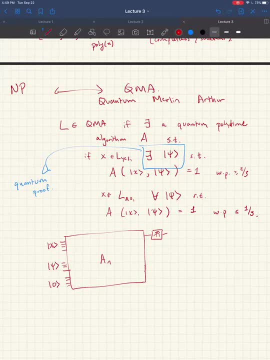 um, and the fact that you know the this proof is some quantum state uh has it makes it have have a lot of different properties, like, for example, you can't copy the proof and share it with your friends, unlike a classical proof. um, you know, due to the no cloning. 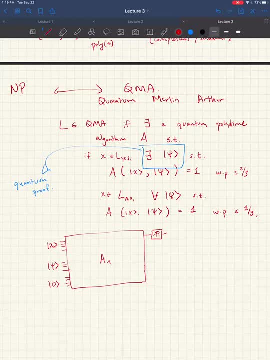 theorem um, it also may be like difficult to extract any information about this quantum proof, uh, other than the fact that this statement x, which you were trying to verify uh, is true or not right, because if someone hands you this quantum state and you try to do some measurements on some part, 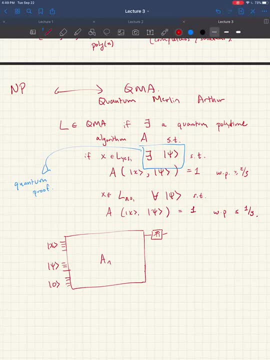 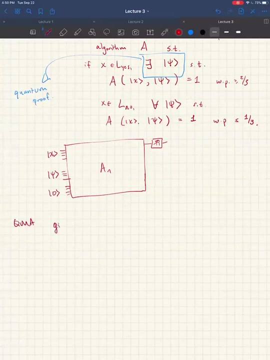 parts of it to try to extract some information. you know the the state as a whole could collapse and and then you would lose information about the state potentially. um, so you know, the point is uh, qma gives rise to a new kind of proof, or a new notion of proof, rather. 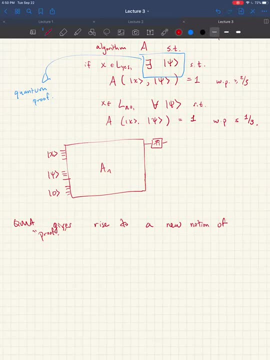 um. and actually this notion of proof expands the realm of things that we can efficiently verify. so examples of, uh, things that can be um, um. so, as we'll see, the local hamiltonian problem will be something that can be checked efficiently using the quantum proof. all right, i'll get to that in a second um. 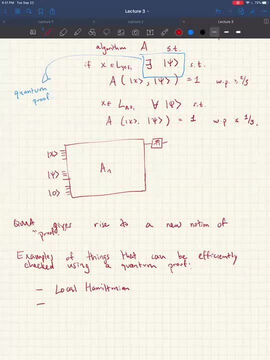 there's, but something that's not related to with these, something called the group non-membership problem. What is this problem? So we all know, you know, hopefully we remember what a group is like in the sense of a mathematical object, right? So a group is some set of. 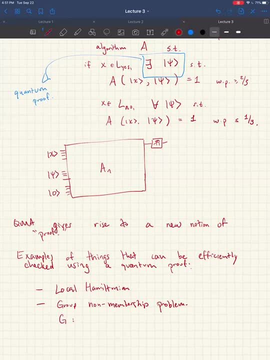 objects, elements that have like a binary operation that we can call multiplication. These set of elements are closed. under multiplication There's inverses, there's an identity element, right? So hopefully you remember this from your algebra class. So the question is: suppose you know someone gives. 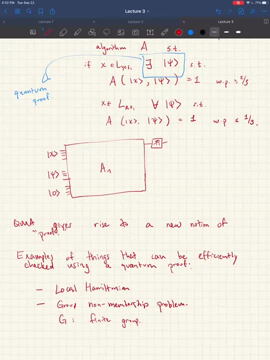 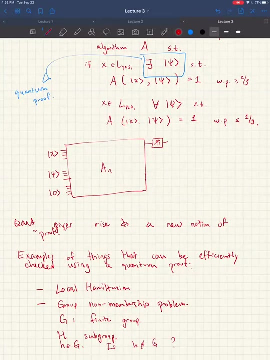 you a finite group in the sense that you like, you know how. if someone gives you two elements, you know how to multiply them together and you can take inverses. and someone tells you a description of a subgroup and then now someone says: here's an element, little h of this group G. Is little h an element or not, sorry, of. 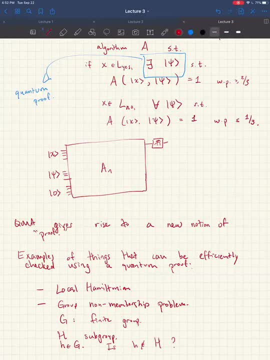 the subgroup H And you have to determine whether that's the case. okay, And this problem, like we don't know how to efficiently like, if this little h is not an element of this subgroup, this seems like a hard thing to prove by just writing down a classical. 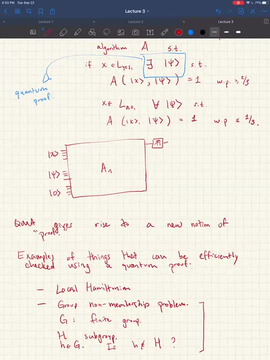 proof right? Basically, how do you show that something is not in this subgroup? Well, you have to show that there's no possible way of of reaching H just by multiplying elements of this subgroup. But it turns out by using a quantum proof you can actually efficiently prove to someone. 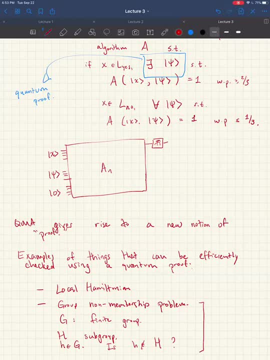 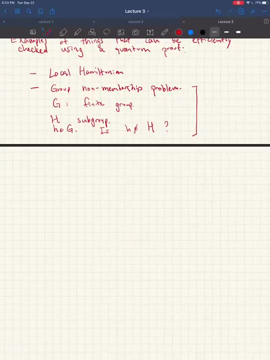 that this is the case. So let me be a little more precise, because this is actually a really cool demonstration of quantum proofs. So So let's say we assume that you have black box access to G, this group, meaning that you have some. 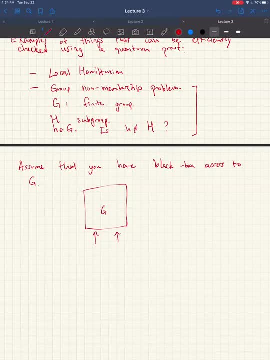 box You can plug in two elements, A and B, and out comes H, the product, a, b. Okay, you don't know how it's doing this multiplication, but it just spits out the product. You can also ask this box tell me an inverse of some element and say, okay, here's the inverse of element a. 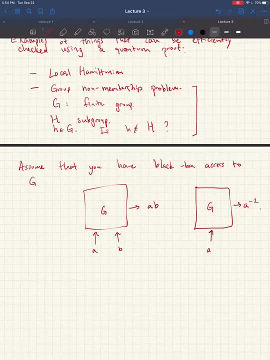 For example, and that's how you have access to the group, And let's also assume that you have some a priori upper bound on the size of this finite group. So you know that s size at most 2 to the n. So this means that 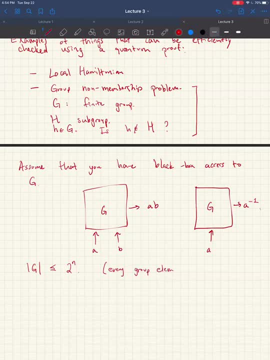 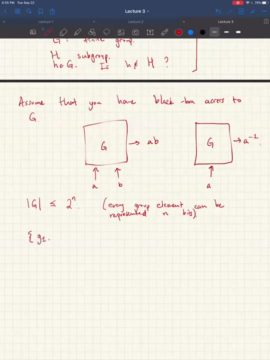 every group element can be represented using, say, n bits. So you can write down the names of group elements. You can multiply them together efficiently Using the access to this black box. So you have this black box and you also have a some set of 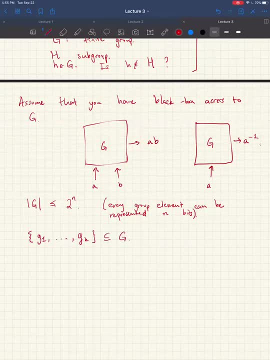 elements of g that you know and someone hands you the set of elements, they generate a subgroup. Okay, so, basically, you take all these elements, You just multiply them by the number of elements. You multiply them by the number of elements. You just multiply them by the number of elements. 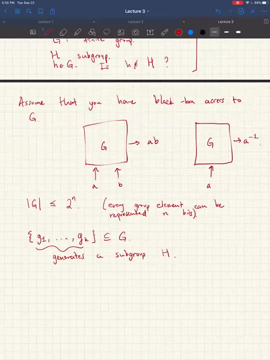 You just consider all possible products of them and their inverses, Right? So you know just diagrammatically, if this is group g, then this g1 up to gk could generate some subgroup of h. that's inside. So and then also someone just hands you some element h in this group. 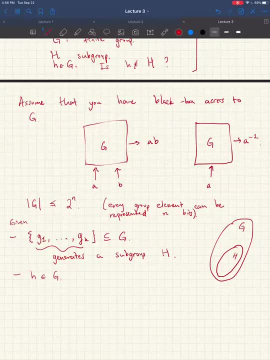 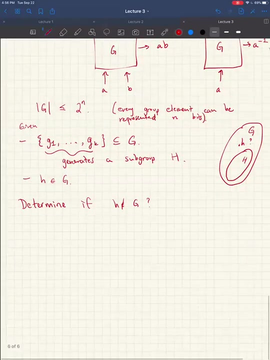 Randy asks: the group does not have to be abelian. That's right. It can be an arbitrary, finite group. It doesn't have to be commutative. So is h and g or not, Don't you mean, is it h and h or no? 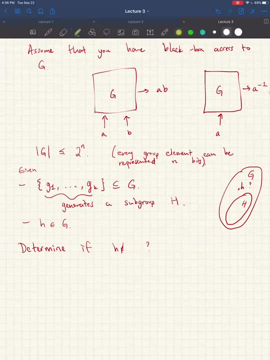 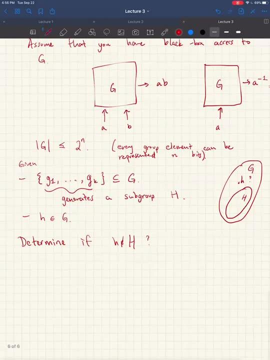 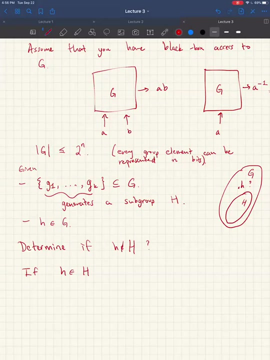 Sorry, I keep on writing. Yeah, it is h and g, Big H in this subgroup. So if h is actually an h, then it is possible to prove to someone that this is the case. So if h is actually an h, then it is possible to prove to someone that this is the case. 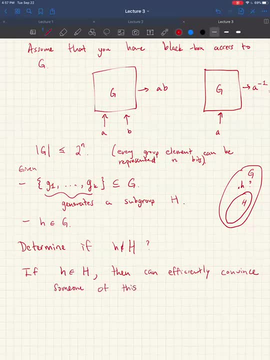 Why is that? Well, there's a study that produced this. Well, surely/ this is a non-trivial fact in group theory, but you know that h is, you know some. you know you can take it in order to generate h. you can multiply, you know, g1 by g10. 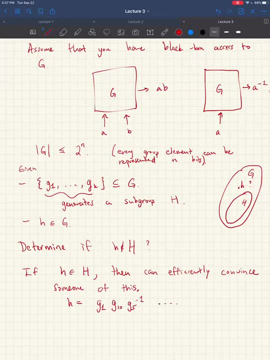 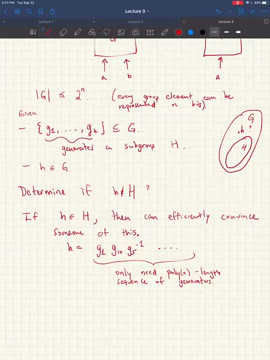 and then maybe g5 inverse and so on. but the point is, whatever product of these generators you have, there's only a polynomial length sequence of products that you ever need to consider. Okay, So you just tell someone, here's the polynomial length sequence of generators. 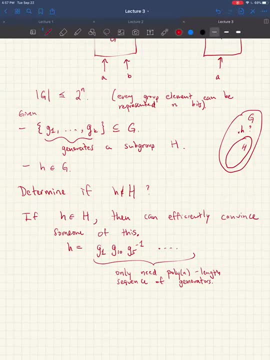 and then that person can use this black box of g to multiply them together and say: oh yeah, it actually outputs h, So that's no problem. Do you know that you only need a polynomially sized sequence? Ah, Um, so it's not obvious? I don't know the proof to this. 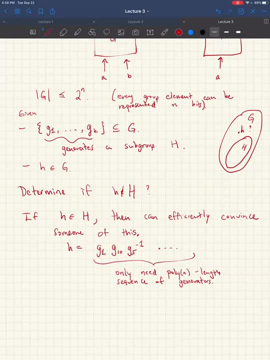 Um, this uh uh comes from um, yeah, it comes from some non-trivial fact in uh Yeah, I think you might rely on the classification of five simple groups, which is very non-trivial. So, uh, yeah, non-trivial facts, Yeah. and then Adrian says this might: 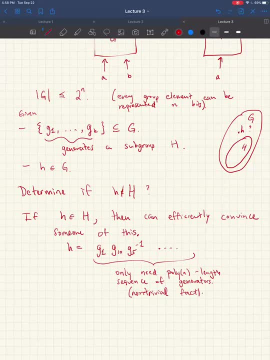 rely on some really uh, heavy machinery. but whatever, it's apparently a true fact. So you know this. this tells us that uh, proving to someone that group membership is is in NP, But here we're actually interested in group non-membership, Right. so it's like proving the non-existence of a sequence of products. 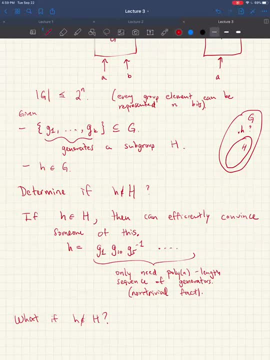 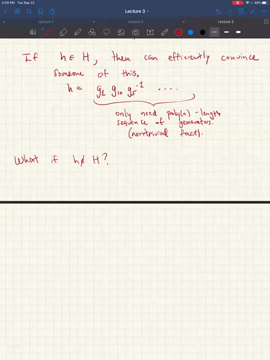 to reach this element. How do you prove non-existence? How do you prove non existence? That's a really weird thing And I'm going to, in the last, like five minutes before the break, I'm going to describe a quantum protocol to do this. 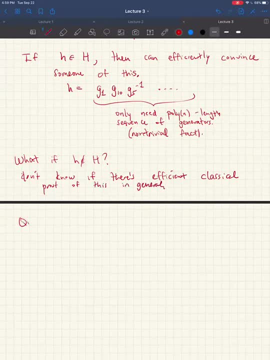 Okay, So I'm going to describe what Arthur the verifier does. so he He's going to get some state from Merlin some side, and we're going to view this side as just some superposition over group elements In G And what we're really hoping. 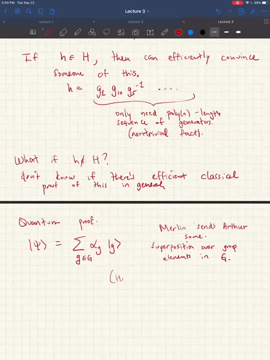 Is that The side is actually the superposition of group elements in the subgroup. Okay, This is what Arthur is hoping, but we don't know that this is the case. Okay, because Merlin- again, he might be devious, He might be trying to trick us. 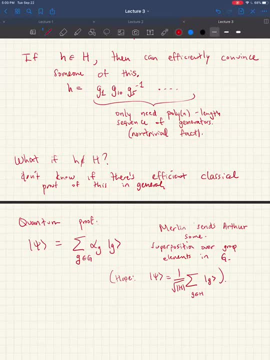 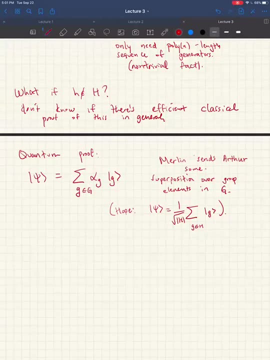 He's just sending us some quantum state, but whatever It's it's, we're going to interpret it as a superposition over group elements. So So Arthur performs two tests, So one test is going to be called the membership test. 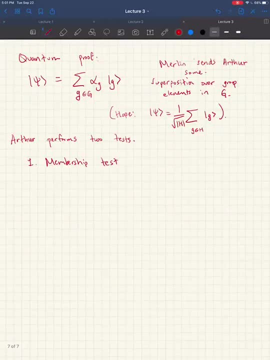 And it's going to be this quantum circuit. So it's very simple. He prepares one qubit in the plus state- This is the equal superposition of zero and one- And he gets. he takes this state that he gets from Merlin and, controlled, on this plus state, he's going to apply a 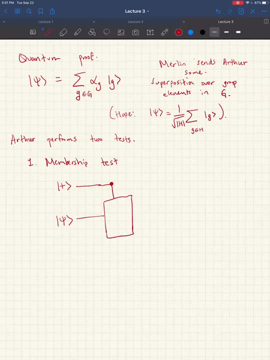 Controlled multiplication by age. So I'm going to call it Okay and I'll explain what that means in a minute. Then he's going to perform a Hadamard gate, And this is not the subgroup H but the Hadamard gate. 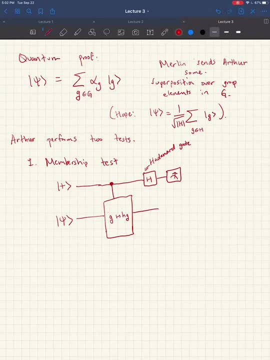 And then he's just going to measure this To determine the answer of this non membership query. And then the other one is he's going to check Whether This side is indeed This equal superposition, Right? So I'm just going to for now, I'm just going to talk about this membership test for now. 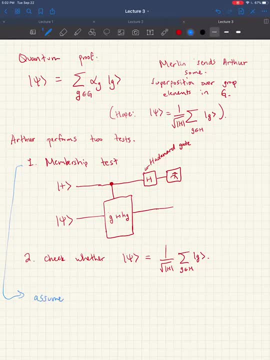 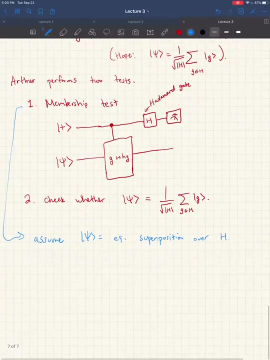 So here let's just assume That actually, sigh, really is this equal superposition over age? We don't know that this is the case, but let's just assume it for now. Okay, Let's see what happens in this, this algorithm. So 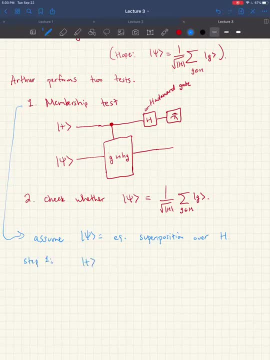 You know, in step one We have This plus state Times, this equal superposition, Right, We do a controlled multiplication. So, Actually, you know what? Let me write this out. So what's the? the plus state is zero and one. 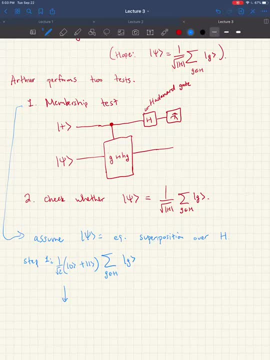 Over two. So in the case that the, the control qubit is zero, We don't do anything. So we have one over root two, one over square root H. Okay, but When the control qubit is in the one state, We multiply everything by H. 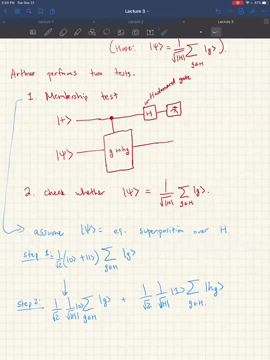 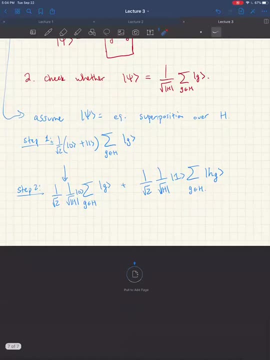 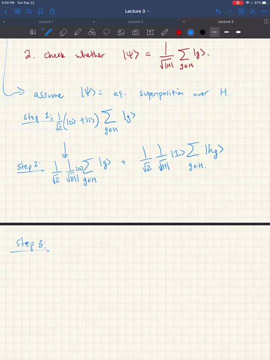 Right. so So we've gotten to this step right now, And finally we're going to do the same thing. Finally, we're going to do a Hadamard gate on the first qubit. So let's call this state- Well, you know, this is state side, as before. Let's call this states theta. 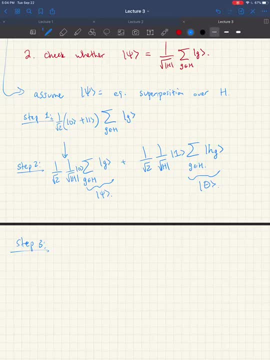 So after the Hadamard gate I'll skip the computation. But what you get is One over root two. Zero tensor Psi plus Psi plus theta plus one tensor Psi minus theta. I think Actually I'm missing a factor of root two. So this is probably a half. 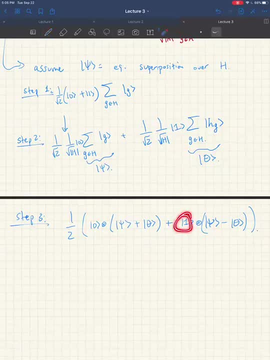 Okay, and then, And the point is, we measure this qubit to determine whether this, This element H, little h, was in the subgroup or not. So here's the claim. We can break it into two cases. Suppose that H was really an element of the subgroup. Can anyone tell me what? 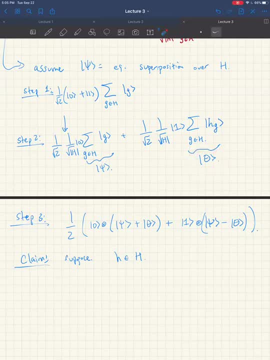 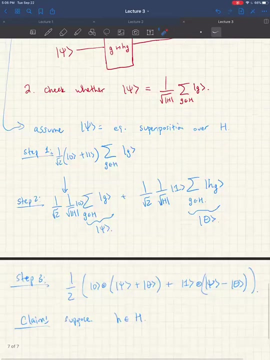 What this state theta looks like. Wouldn't that just be psi? Because if you multiply elements of a group by an element of that group, it just Identity gives you back to the subgroup, Exactly So. So here, where was my diagram? 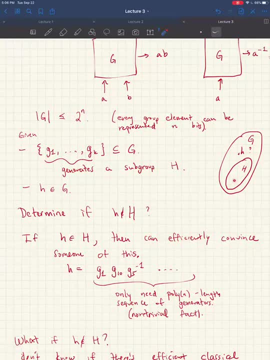 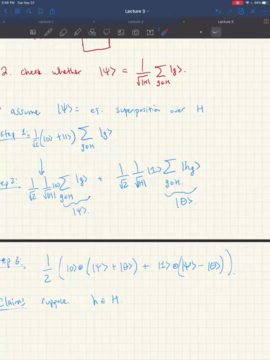 So here H, we're assuming that H is part of this big H. So if you multiply everything in big H by H, it just sort of shifts everything around, but you haven't moved outside of H, of capital H. So so this is still, as Hugh said, an equal superposition over elements of H. 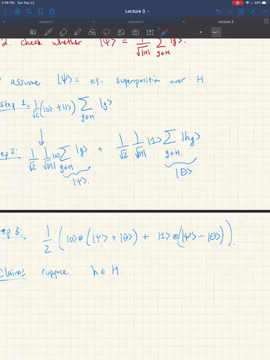 So what happens is that the psi minus theta is equal to the superposition over elements of H. So what happens is that the psi minus theta is equal to the superposition over elements of H. For now, the data is going to be zero. 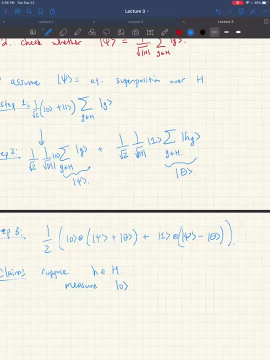 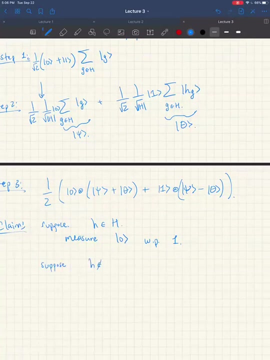 And then you're going to measure ket0 with probability one. So the algorithm has correctly identified the no instance. So now suppose H was, was not a member of the subgroup, then what can you say about the relationship between psi and theta? So first question: are there any overlap between the elements? 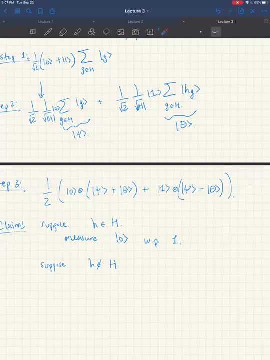 of here and the products here. No, They're completely disjoint, right? If you take a subgroup and multiply it with an element that's outside the subgroup, you're going to completely shift that group. So psi is orthogonal to theta and then you're going to measure one. it turns out with probability of half. Okay. 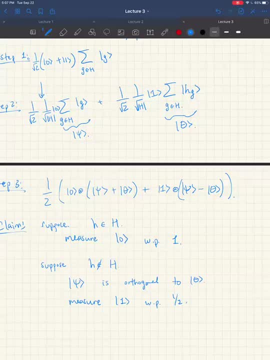 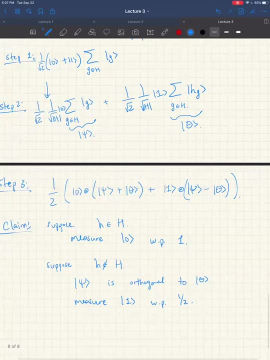 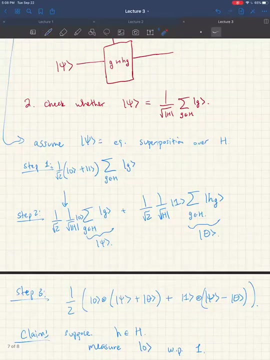 It won't be 100% certain, but you at least get one with probability of half. So at least in this case, where we're assuming that psi was really this uniform superposition over H, your algorithm has some noticeable bias in terms of determining what 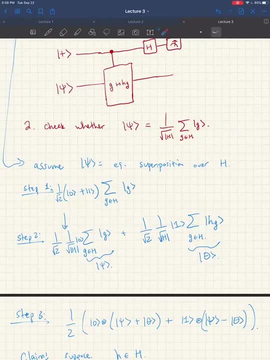 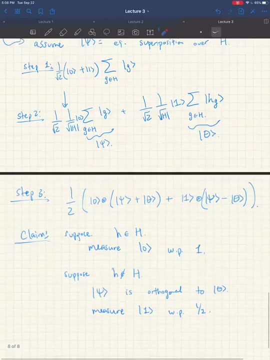 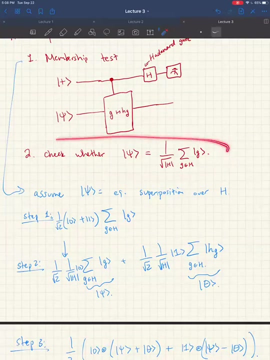 the right answer is: Okay And good, So we're almost done. The only thing is: well, how do we? We have to check how. How do we actually have this uniform superposition? And this again uses some non-trivial results. 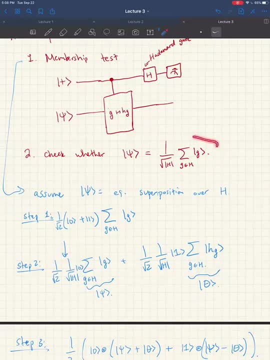 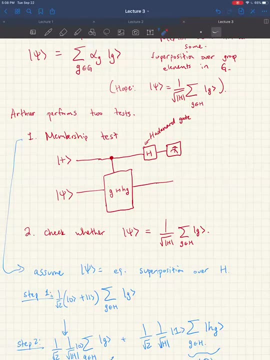 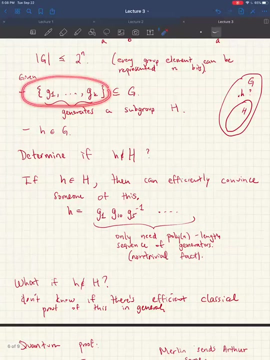 in group theory. If someone hands you a state, an arbitrary state, you can test whether it's And you have the generators of this subgroup. You know you have the generators of the subgroup. You can test if the state is the superposition over that subgroup. 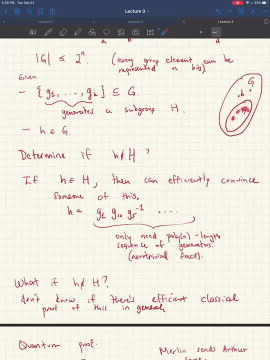 First you generate a random element of the subgroup- which is possible to do in polynomial time- And then you just basically multiply the state with that random element and you see if it leaves the state invariant. Okay, So I'll just write that down and we'll take. 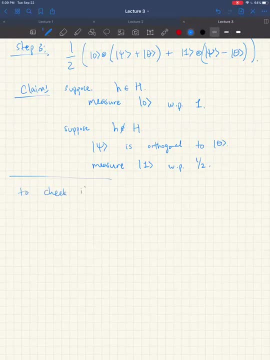 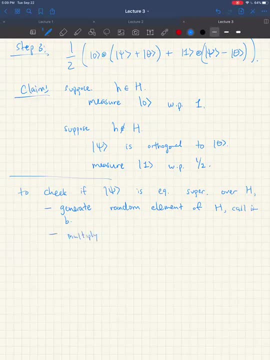 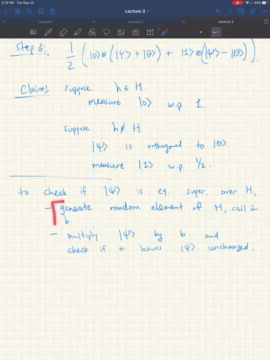 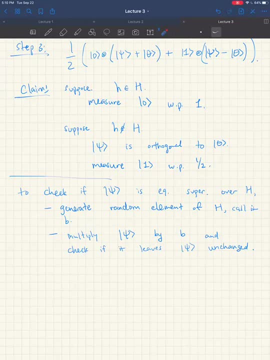 Yeah, Just back to the definitions of BQP and QMA. Are we allowing x to be quantum as well, or does x have to be classical? Here x is classical. Would it make a difference if we allowed x to be quantum? Super great question. 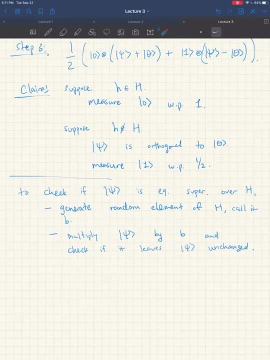 So people really haven't formulated a theory around that. So far, people focused on classical inputs x because they want to relate it to classical complexity theory, in which case the inputs are always classical. But actually this is something I'm interested in, which is like: can you? 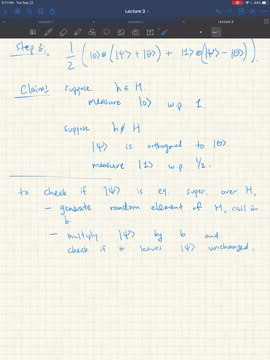 define a complexity? Can you define a complexity theory with quantum inputs, Where you have decision problems that are sets of quantum inputs? So if people are interested in thinking about that, I'd be happy to talk about that. Could you just go over again why, if h is in the subgroup? 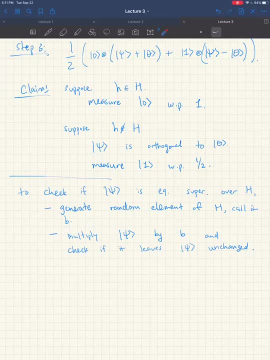 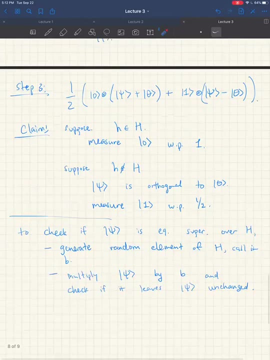 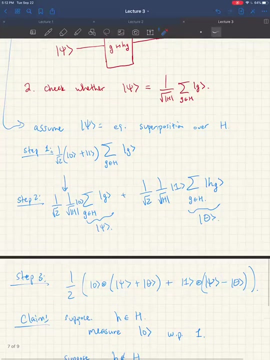 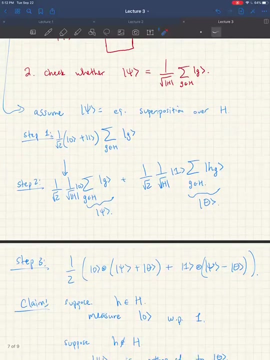 but not x? Yeah, So you're saying that theta and psi are equal? Sure, Yeah, So where were we? Yeah, So the question is- This is the first claim, The first claim. Yeah, So this is theta, right. 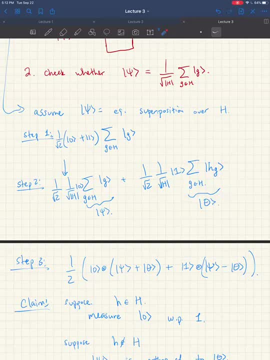 Yeah, And the question is: well, what do I mean by hg? Yeah, Well, I mean so h and g are group elements of this mother group g, And then we're going to multiply them together. So this hg is going to be a label of a group element within the mother group. 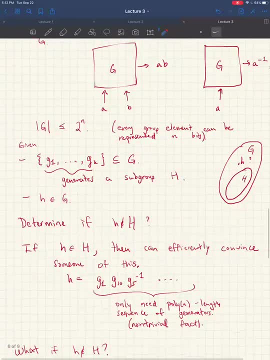 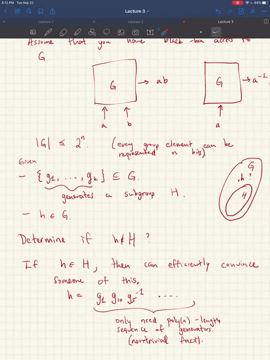 And then the way we multiply it is by using this black box. So we plug in h here and then we plug in g here, And this will tell us hg. Cool, But we know that hg is going to be an element. It's going to be an element of h. 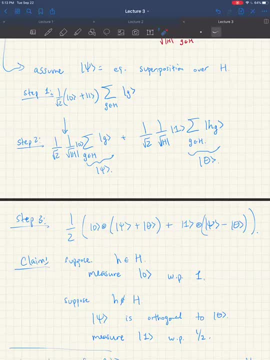 Yes, Okay, Yeah, I got it. Yeah, And so it's also like a bijective map. Yeah, Yeah, I see, Yeah, Thank you. And when you say efficiently convince someone here, is that like polynomial, with respect to k, being like the- or with respect to n? 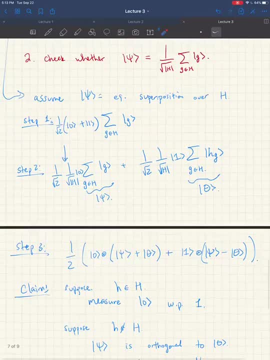 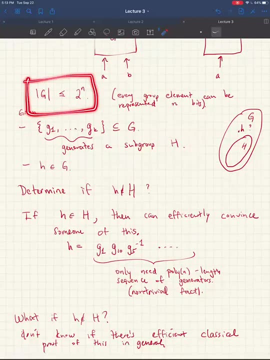 Or what is it? Oh great, With respect to n. Yeah, So here there's- we have some parameter n which just gives us an upper bound on the group g. So I mean polynomial in n, Because, like that's- we need n bits to write down each of these things. 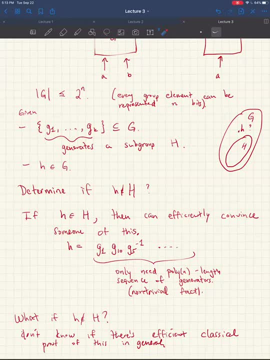 And all of our computations are polynomial in little n. Thanks. I have one question: Do we know for sure that this problem is not an NP? No, not at all, It's still- it still could be an NP. I mean, of course, with anything in complexity theory, like lots of things could be in P. 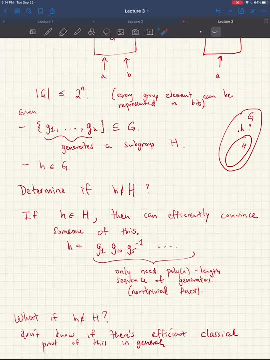 Right, But we don't know. I think the best upper bound we have on this is- I'm tempted to say it might even be in QMA. Oh, wow, Okay. Yeah, I think Lassi-Babai believes that it might be in classical MA. 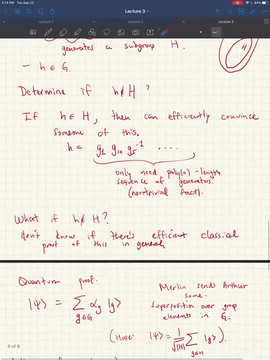 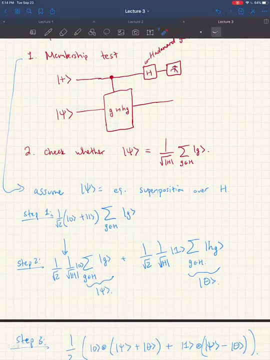 But as far as I can tell, this might still be an open question. Okay, Cool, Henry, Mm-hmm, Could you clarify something for me with the definition of QMA? Sure, So when you say that if the instance is a member of the yes class of the decision-making? 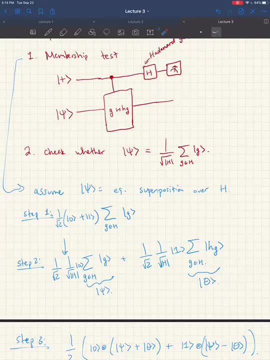 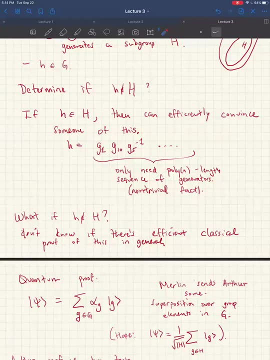 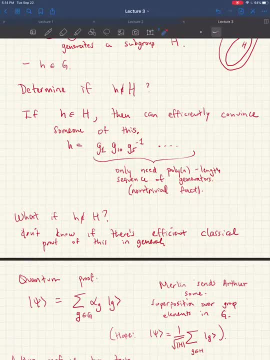 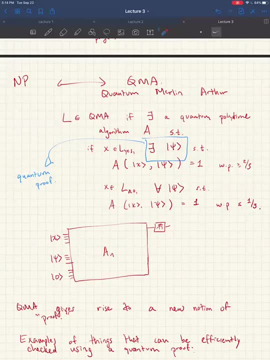 Right, So it's not an NP, Right, Right, So it's not an NP for the decision problem: Mm-hmm, And A returns one with a certain probability. So is that probability reflecting the membership of the instance as a yes instance, or could? 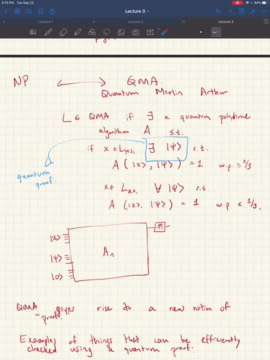 you interpret the probability as to do with whether the proof is actually a valid proof of that instance, Or is that I would say it's more like the latter. It's, I mean X, is It's, either in. it's either yes instance or it's not Right. It's whether it's how convinced. 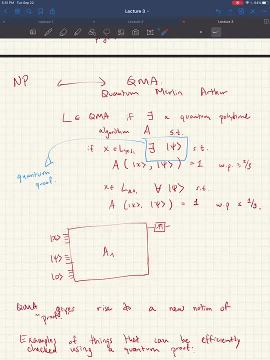 this algorithm is So. so you know, think of it this way, like you know. just maybe this where the personification helps: like you know, imagine you're the algorithm. you get this quantum state at psi, you do some computation, then you measure, and then it outputs one, and then, and then you say: well, is it more likely? 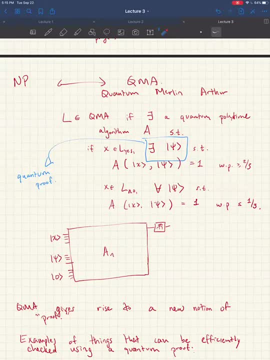 that X is a yes instance or X is a no instance, And then, because of these numbers, you should two-thirds versus one-third. you should say: well, I you know more convinced that it's a yes instance because it's more likely. Okay, thank you. 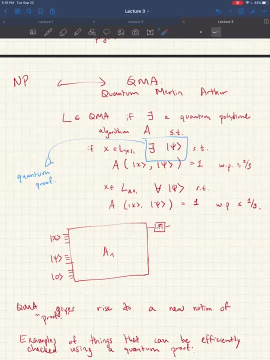 And then protocol. Oh, I see Also, Adrian, you sound like Darth Vader. Oh, is my mic not working? It's very, very scratchy. Okay, I'll try to figure out what's going on. Sure, I see, but yeah, I guess Adrian said it's it's an AM, which I guess that's. 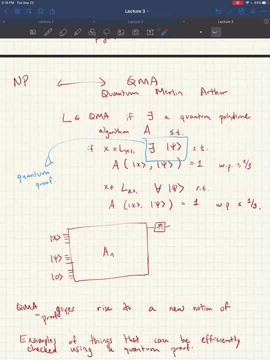 incomparable to QMA? It's an interesting question. It's an interesting thing, You know, let's see. Randy asked I might be missing something, but the quantum proof does not depend on the little h. Yes, the quantum proof only depends on the subgroup of big H. Well, in this, in this analysis, we're assuming 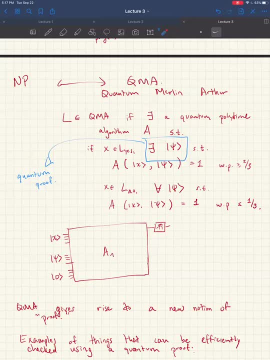 that Merlin is is being nice and telling you the right thing. In the adversarial case Merlin can give you anything, but we have a this extra test to check that he's he's giving you the right kind of proof state. Yeah. and then Hugh says, yeah, that what? what? the verification algorithm does it. 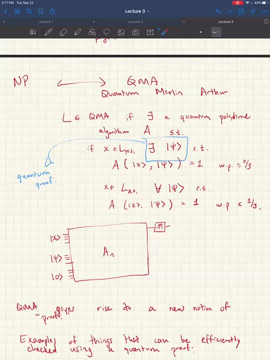 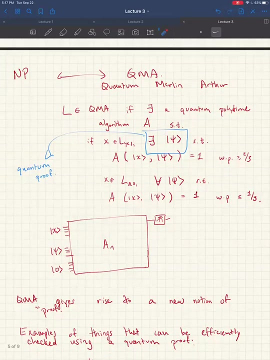 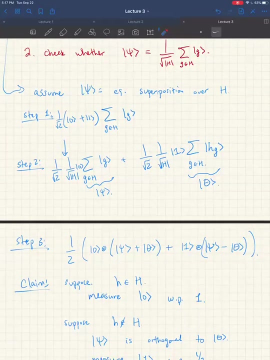 will do something that depends on little h- Great questions, Okay, so maybe let's let's continue on. So this group non-membership thing is kind of cool because it's like groups and you know membership of elements and groups. this is something that comes from like abstract algebra. 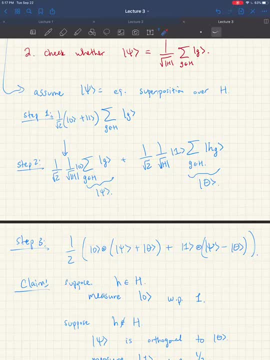 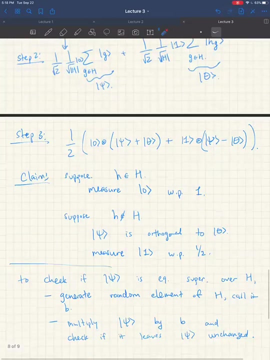 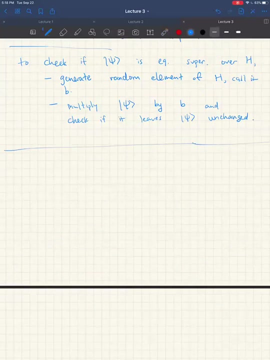 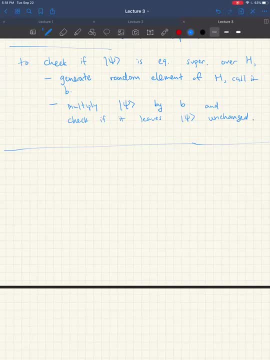 Okay, Okay. And just another comment about, like You know, you look at this saying: well, where is the Quantum advantage coming from? describe n qubits. you need a two to the n size classical description. You need to keep track of exponentially many parameters to describe this quantum. 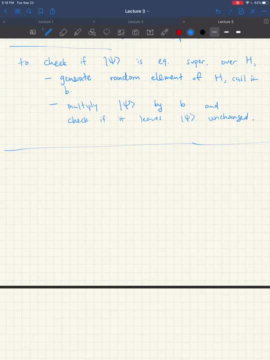 state. So maybe that's why, at least in this group non-membership problem- Merlin is able to convince you with a quantum proof, because he's packing in. maybe he just takes an exponentially long classical proof and squeezes it into an n? qubit quantum proof and somehow that's what's happening. But 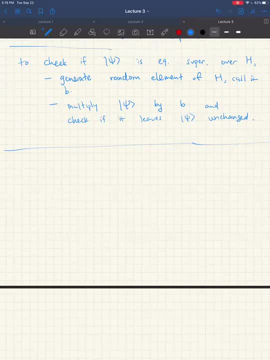 that's actually. that would be kind of like the wrong intuition to take away. because you know, even though an n qubit quantum state requires exponentially many parameters, you cannot reliably store an exponential amount of information in n qubits. Because if you try to do that and you 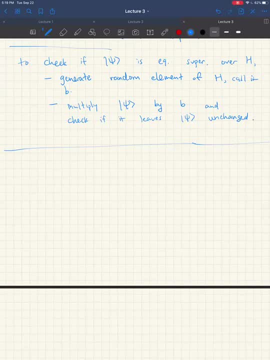 sent these n qubits to someone and they try to uncompress or recover that exponential power. they can't store that information. So you can't store the amount of information. they would make some measurement, but then the state would collapse and all that information would just disappear. 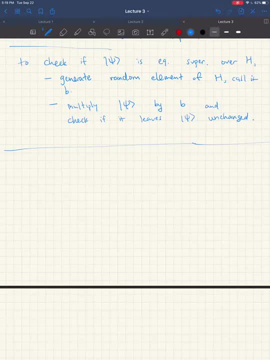 So quantum states are fragile in that way. In fact forget exponential If you have n qubits. there's something known as Halebo's theorem that says you cannot reliably transmit more than n classical bits of information using n qubits. So this advantage in verification for the QMA setting is coming from something else. 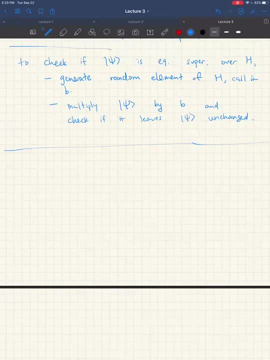 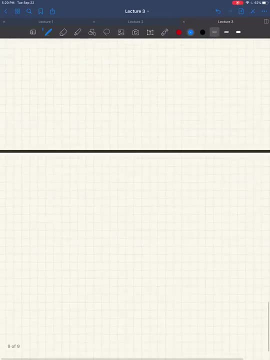 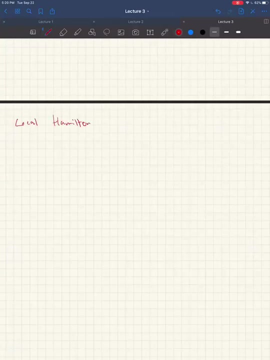 What it is. I don't have a much better answer, but it's definitely not just squeezing in classical information in this naive way. So let's go back to local Hamiltonian. so we'll go back to quantum physics And we want to show that this local Hamiltonian's 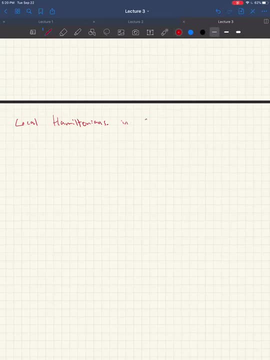 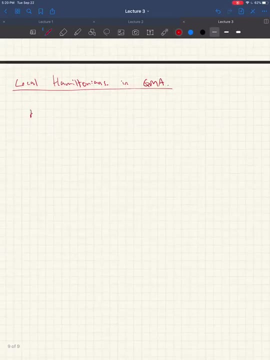 problem is in QMA. So we have this k local ham problem, We have these parameters a and b, So suppose someone walks up to you with an instance of this. So they have a local Hamiltonian and they're claiming the ground energy. 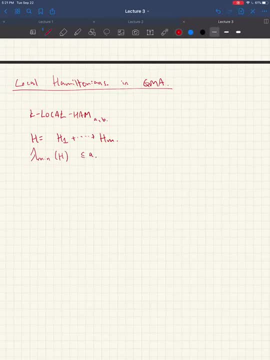 of this Hamiltonian is less than a. So how might someone convince you of this fact? Give you an eigenstate? Yeah, well, in particular, which eigenstate? The ground state, Yeah. So Merlin can say: well, look, here's the ground state. 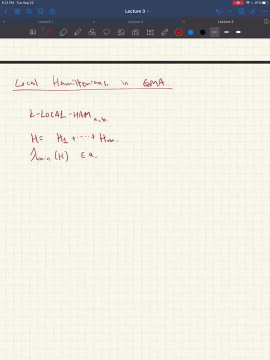 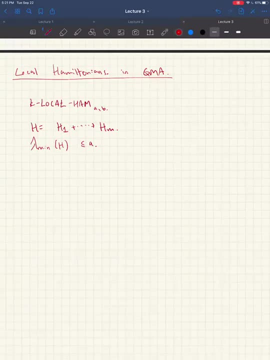 This thing certifies that the energy is less than a right. And this is again where Where quantum helps, because if Merlin was only able to give you a classical piece of information, it's not clear how he could do that other than just writing down all two. 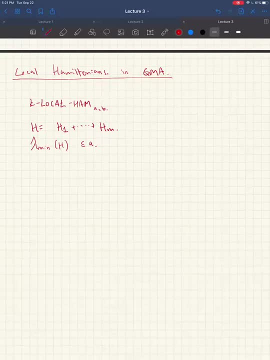 to the n amplitudes of that state, which would be too big. But giving it, Handing it to you in quantum form, you can actually do something efficient to check. You want to check. Yeah, Yeah, Yeah, You want to check if this proof, state h, really has low energy with respect to some. 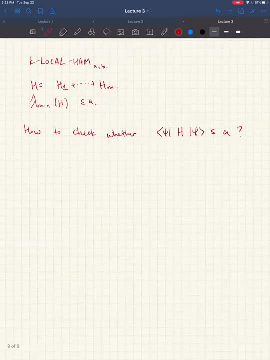 local Hamiltonian. So how do you do this? Well, let's sort of just write out, expand out the definition of this energy. So this is equal to well. we have a bunch of local terms right Each h? i. 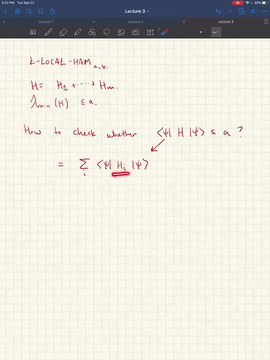 This is where locality comes into play. h i only acts on k qubits, So think of k as being like two or three qubits, right? So you really just have to measure. So for each term, i measure the energy of psi with respects to that local term. 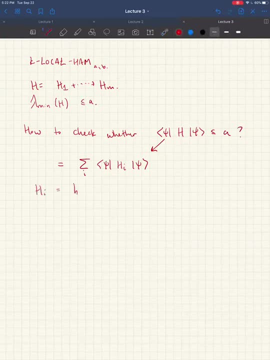 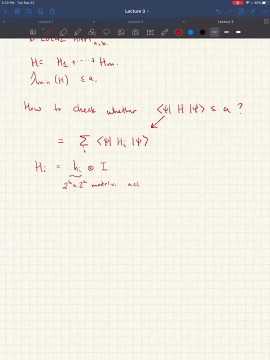 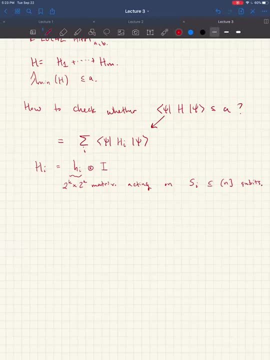 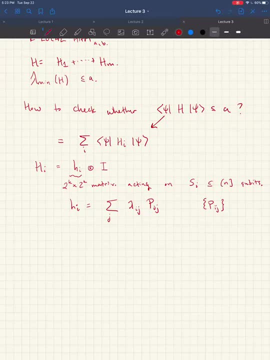 form a projective measurement. right, because they're orthogonal, they sum to the identity And it's a projected measurement on k qubits. So again, just continuing to expand, We get that this is equal to sum over i, sum over j. 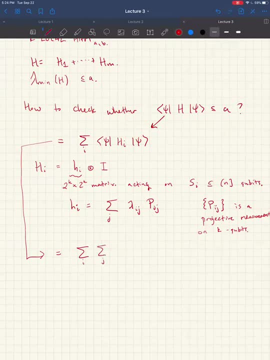 We have lambda ij Sum over i, sum over j, Pij, tensor identity, Okay, and we can think of: You know again, like this is sort of your kind of like You know, for each term i, You're doing a measurement on some small number of qubits k. using this projected measurement you get outcome j with this probability. 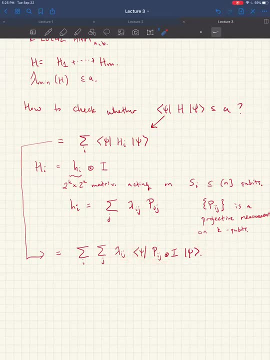 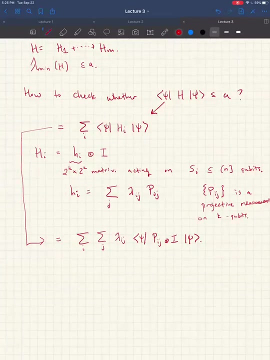 And then you output An eigenvalue, lambda ij. Okay, And so this is the quantity that we want to estimate efficiently on a quantum computer. So you know, this suggests the following algorithm: So step one of the algorithm: Let's assume for now that the input is some large number of copies of the supposed ground state. 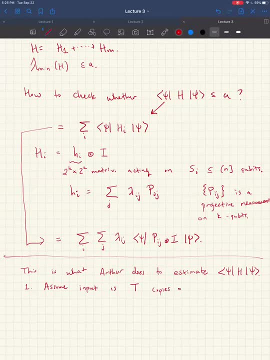 Let's call it some large number, t. Okay. So step two: we're going to have some counter that just keeps track of our energy, And then we're going to do the following many, many times. So for t equals 1, up to big T, we're going to pick a. 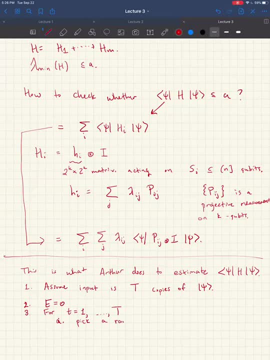 random term to measure. So we have an m-term Hamiltonian. we'll pick one of them at random. We're going to load a fresh copy, one that we haven't used yet. fresh copy of psi. We have many copies of psi, let's just 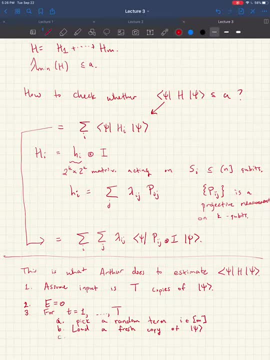 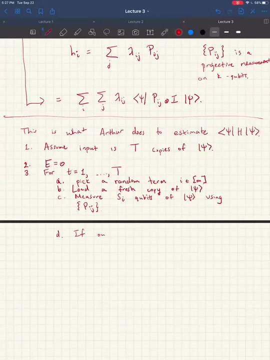 take the one that we haven't used yet, And then we're going to measure the SI cubits of psi using this projective measurement, pij, Which we have defined up here. It's like the projected measurement corresponding to the i-th term, And if the outcome is j, 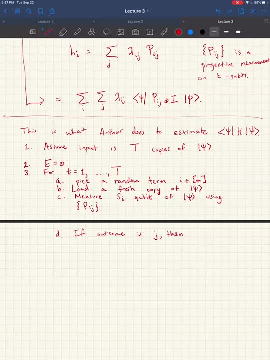 then we're going to set some random variable x sub t equal to the this corresponding eigenvalue and we're going to just multiply it by m, just for reasons that you'll see later. Okay, so for every little t, we're going to do this measurement and we're going to get a sample of this random variable x sub t. 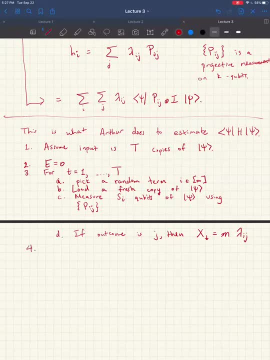 So we do this like a gajillion times and at the end we're just going to take a large average. So, out of all the random variables we've collected, we're just going to take this average and that's going to be our estimate of the energy. 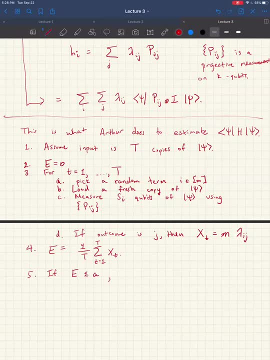 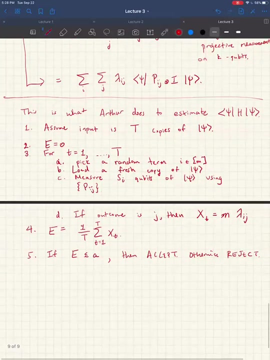 If this e is less than a, then we accept, otherwise we reject Any questions so far about the description of this, This verification algorithm. I have a question. So all these T capital T copies of psi, those are given by Merlin right. 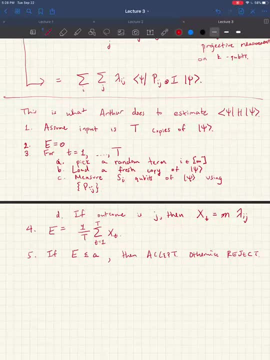 We're assuming yes, So how do we know that he's giving us identical copies? I think I want to relate this question to something I was wondering before, Which is when defining bqp, we said that the thresholds two-thirds and a third are. 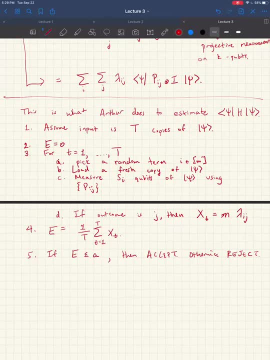 arbitrary because we can just repeat the algorithm many times. But that doesn't seem to be the case- or maybe I'm just not seeing it- for QMA, because for QMA to repeat the algorithm many times you would need many copies of sign. There doesn't seem to be a way to both check that. 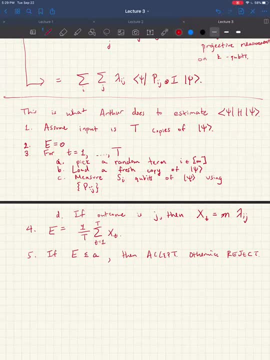 the copies are the same and use them. That's a fantastic question. So I guess comment number one is: you're absolutely right. It's not obvious that you can just repeat with QMA to amplify the success probability in the same way that you would just do it for BQP. You can, but it requires 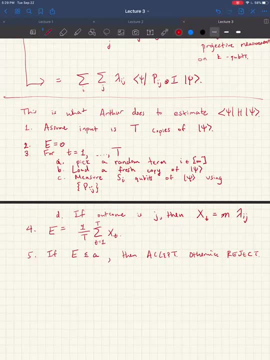 some arguments and I might have a chance. it might even be like a problem set question. Comment number two is: you're saying: how do we know that Merlin is handing us T identical copies of the same state? Right like you know, we're thinking of Merlin as being someone who's trying to make our lives. 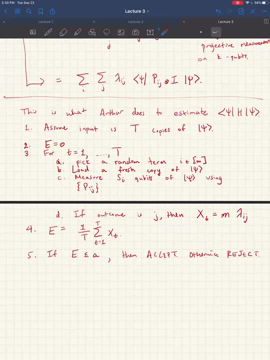 difficult. So instead of handing us T copies of state, you could just hand us some arbitrarily complicated entangled state across T registers. That's possible. It'll turn out that it doesn't help Merlin to do this, But just for now, just to make things simple, let's assume that 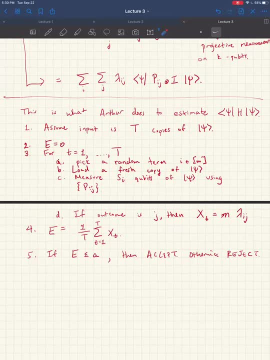 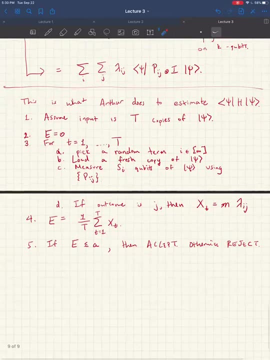 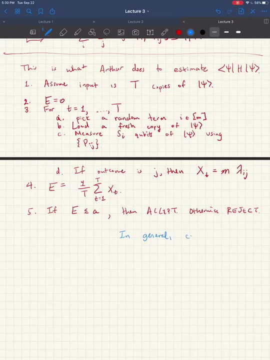 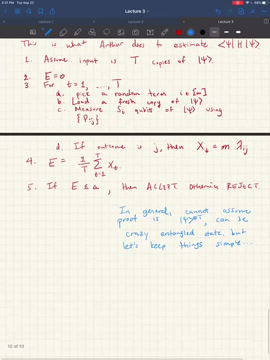 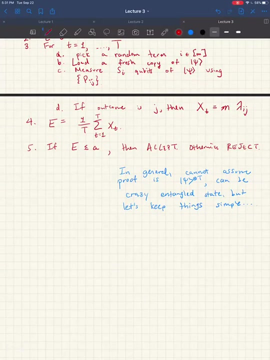 we really do get fresh copies of, you know, IID copies of this. So that's a really good question. In fact, I'll make a note of it Okay. So let's yeah any other. so before I like analyze why this could be a good 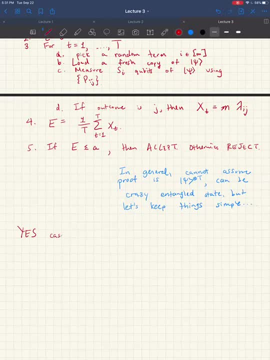 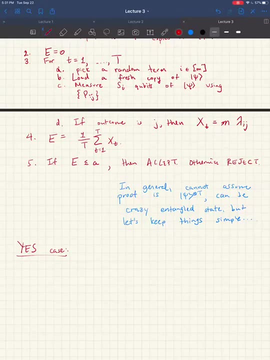 verification algorithm. any other questions about, like, the definition of you know this algorithm or what's going on, So like, if like, so for every. let's say for every, because you're randomly picking the terms. 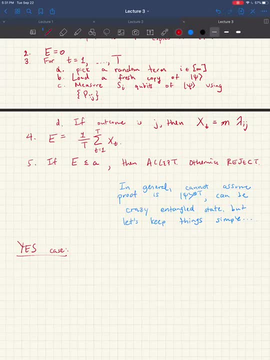 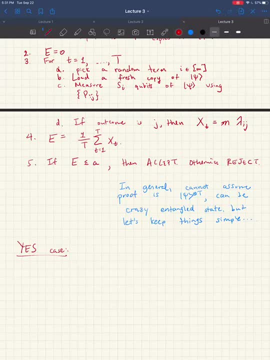 Because if you haven't, you cannot, it's not the full eigenstate of the Hamiltonian right, Because you might be missing a term or something. So how do we Right? So the way to take care of that problem is to ensure that t is large enough so that with 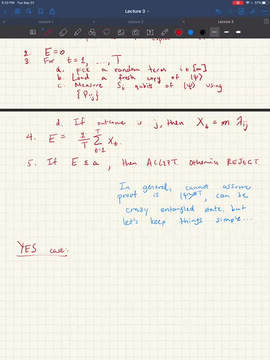 very, very high probability. you've covered all your terms, Okay, So let's say, let's say t is like m squared. then I mean it's vanishingly small probability that you won't sample all the terms. 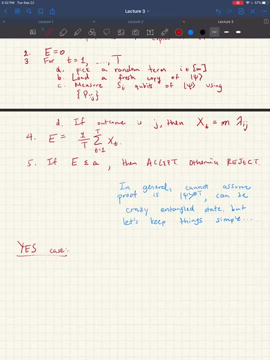 Okay. so like it's more of a probabilistic argument that, okay, we will at least have it once And then okay, And not just once. but you know enough times to to get your estimate correct. Is j chosen randomly as well? 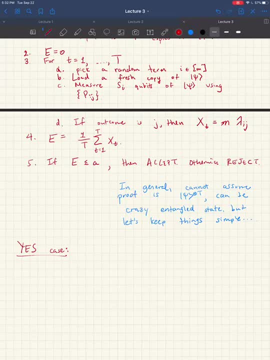 It's random because of the measurement. So so this, this, this projective measurement, this pij, has outcomes indexed by j. So when, so you do. but this whole set is indexed by i. So when you do the ith measurement, it outputs a j with some probability. 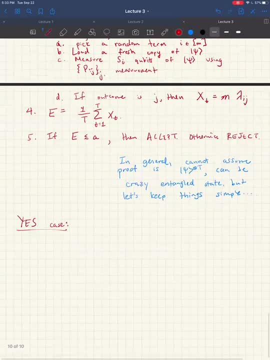 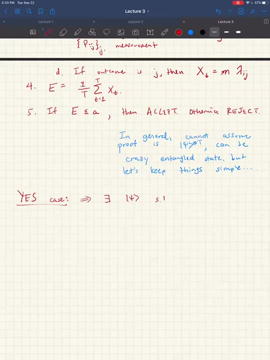 Okay, Yeah, In fact we'll. we'll see it with this analysis right now. So so let's assume we're in the yes case. That means there really does exist a psi, such that: Okay, Okay, Okay, This energy is less than a. so Merlin will say: okay, I'm going to hand you a bunch of 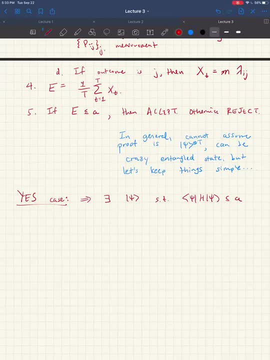 copies of this side right? So let's just look at this random variable. What is its distribution? What is its average? Well, let's just focus on its average. So X of t. well, you know the, the average is. 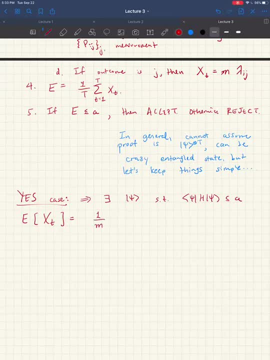 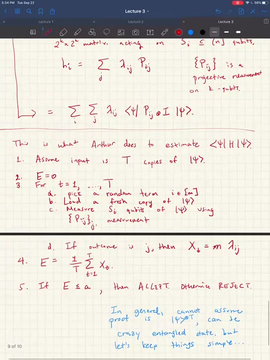 going to be. you picked a term uniformly, at random, between one and m, And then you measured psi according to this projective measurement, pij, right. So what does j run run up to? Well, it's, you know, this little hi is dimension two. 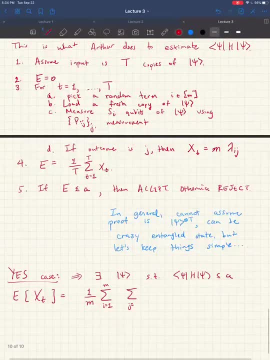 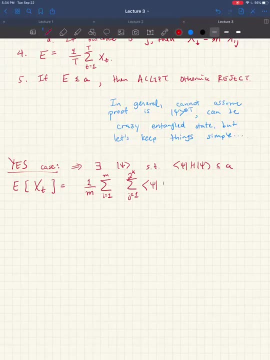 to the k by two to the k. So that's how many j's there are. Okay, Okay, Okay, Okay, Okay, Okay, All right, All right. Well, if it's such an intelligence wrought, right? So this is the probability of obtaining the jth outcome. 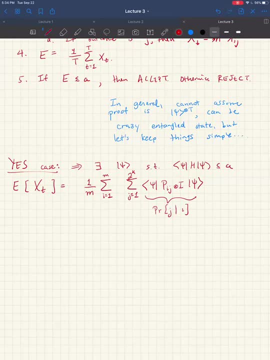 Given that your term is the ith turn. Once you get that outcome, your random variable is going to take on value a. Lambda ij times M. okay, According to my definition, but you know this should look very familiar. The m's cancel. 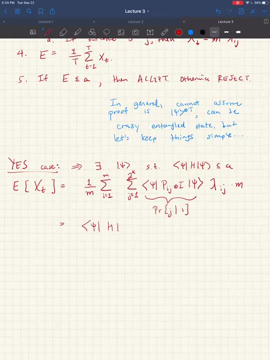 And I claim that we just get this energy of psi with respect to a, j Right. It is absolutely arbitrary. There is nothing to the short right psi with respect to H, which is the thing you wanted to estimate. so it's very good. 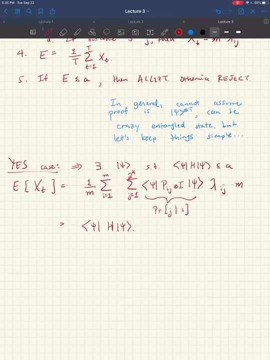 that this random variable has its expected value is the the number we really want to estimate. and we're drawing T samples of this IID, of this same random variable, and we're taking an average right. so it should be very believable that as T goes large by it, like you know, standard concentration arguments or law of large, 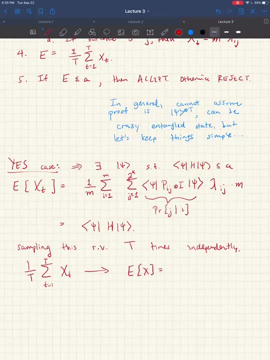 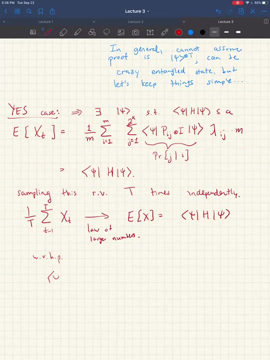 numbers, this is going to converge to the expected value, which is right. so in, in fact, you know, with, with very high probability- and you know I won't say the exact bounds here, you know you can work them out- we'll have the following guarantee that this average will be, you know, within plus or minus. 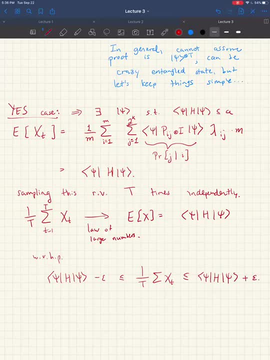 epsilon of the true number you want to estimate. okay, and by taking, you know the exact number you want to estimate. and by taking T's to be some sufficiently large number- that's polynomial in the number of terms, you have, the number of qubits- we can guarantee that this epsilon, this 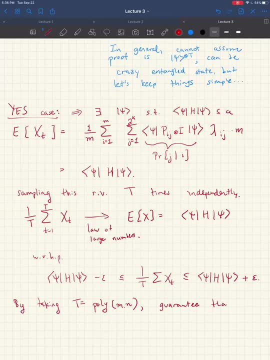 like precision, is going to be much less than the difference between B and A right, which is the gap you're trying to distinguish. so you know, once you've guaranteed that you're going to be able to estimate, that you're going to be able to see this point, then your estimate will tell you whether you're less than a or 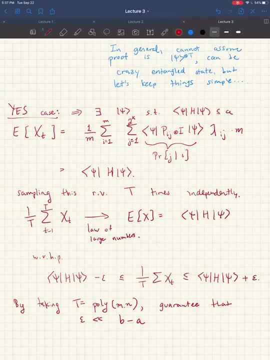 below less than a or above B, with with high probability. okay, so that's you know. so hopefully that should make a lot of intuitive sense. I mean, you're you're just making these local measurements randomly, but you're doing enough of them to estimate the, the global energy, with high confidence and high precision. any, 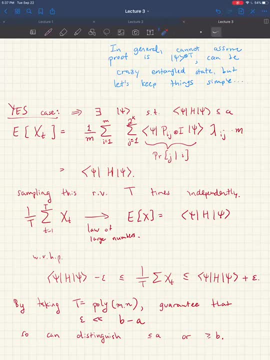 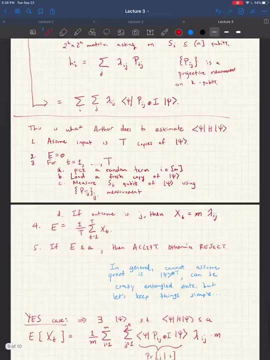 questions about this so far. so the runtime also be polynomial in like one over B minus a? yes, that's right. so I mean that basically comes into what T is. so T actually also depends on b minus a. so actually I think I forget. Sorry, I think I forgot to say something about this local Hamiltonians problem. that's kind. 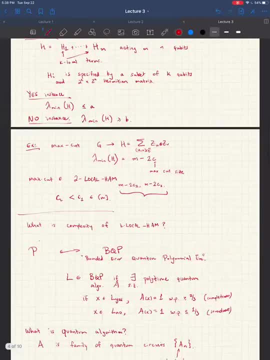 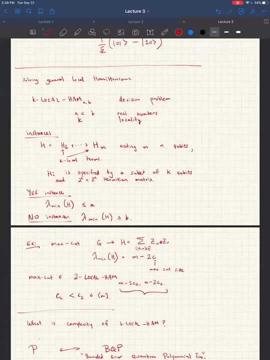 of important for this, and it's also related to your homework problem. We also need to assume that each of this is- and this is just for like normalization purposes- the operator norm of each of these terms individually is at most one. The largest eigenvalue of each of these terms is at most one. 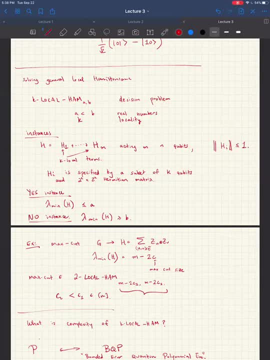 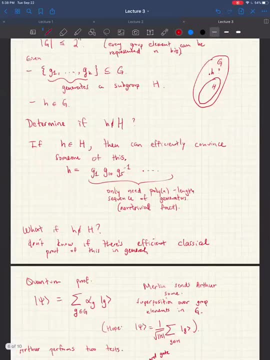 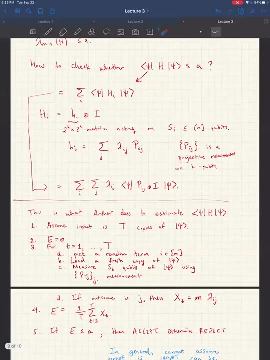 So this is just to ensure that, like your scale, for which your energies live at, aren't like off the charts. Or to put it another way, it means that these lambdas are between minus one and one, So you have some reasonable bound on what these lambdas are. 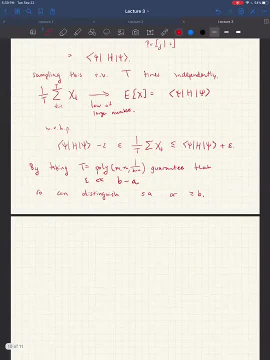 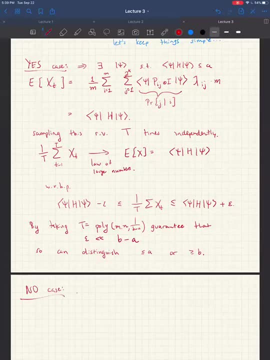 Okay, so that's the yes case. So if there really is a low energy eigenstate, Merlin can convince you of this fact. What about the no case? And if Merlin actually gave you, you know, T copies of some state psi, it doesn't matter. 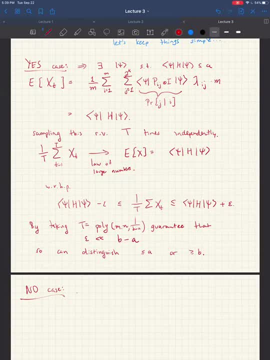 what state? because we know that all states have energy at least b. Okay, So that's the yes case. So if there really is a low energy eigenstate, Merlin can convince you of this fact- What about the no case? Then you know, your algorithm will still work because it's going to estimate the energy. 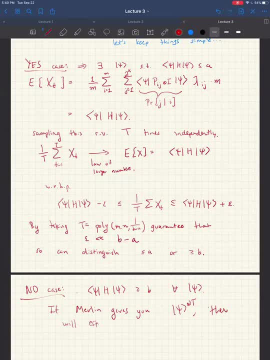 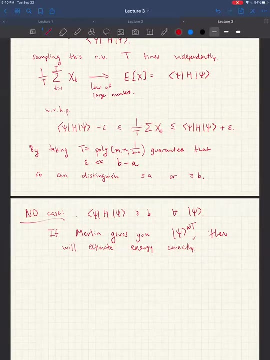 correctly. Well, what if Merlin doesn't give you, Uh Yeah, what if Merlin doesn't give you T copies of psi, but it gives in mixes and matches, like for different coordinates. It gives you, You know, you know, psi 1 and psi 2, tensor psi 3. 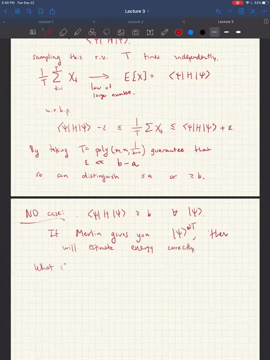 Anyone have an idea what happens then? Well, I don't just, in expectation, get the average of their energies- yeah, like their energies, Which, if they're not all the ground state, then it'll be at least as big as the ground state energy. 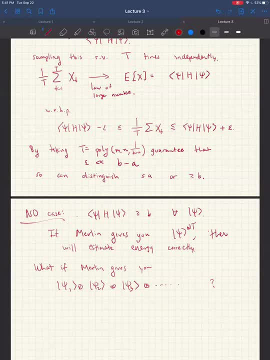 Mm-hmm. So if you're with, the ground state is higher than B and you take the average of a bunch of Or in expectation you get the average Of a bunch of things that are higher than your ground state, then expectation will get something higher than B. 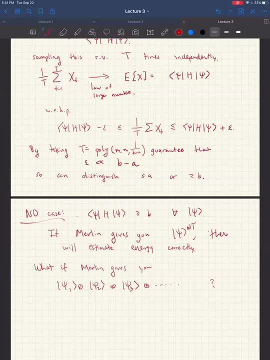 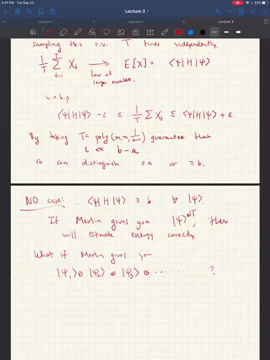 Exactly So it you know. Merlin can't convince you otherwise because you know each of these random variables. They might have a different distribution because you're using a different side each time, but the average is always going to be above B. so So this is still fine. 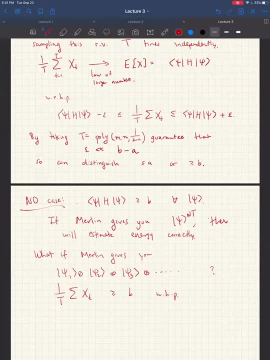 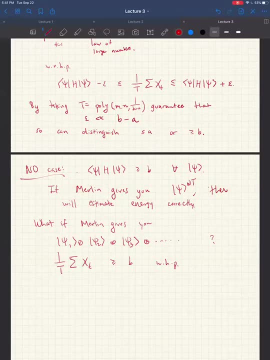 Arthur Will be like: okay, it's not less than a. the more nefarious thing is, if you know, Merlin sends a giant entangled state that's not necessarily like a. you know a bunch of tensor copies of states And the. the claim is that It still doesn't help Merlin. like it actually, your algorithm will still realize that the, the ground energy is, is at least B. 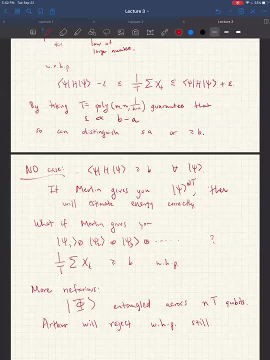 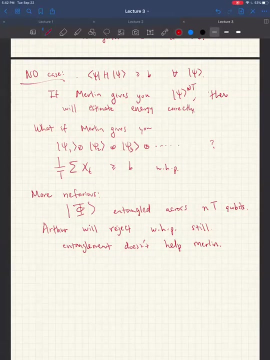 But this, you know, this requires sort of a little more intricate analysis, but it but it is true like this entanglement doesn't help, Merlin. Okay, So this shows, You know, basically we've just seen module on this. This last part is that this kale, A local Hamiltonians. 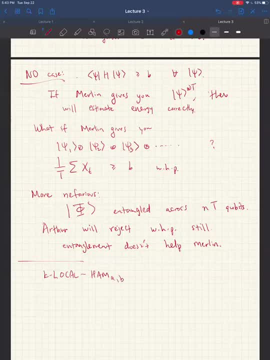 Hebe isn't QMA As long as be minus say is not too small, so be minus say has to be simple, insignificant, to be separated by at least some polynomial gap. Okay, so so far, so good. We followed this classical quantum dictionary pretty well. Local Hamiltonians are quantum analogs of CSPs. 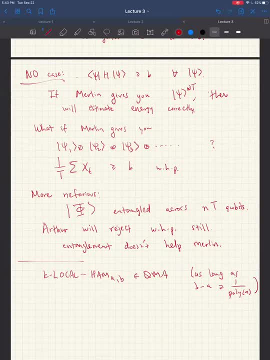 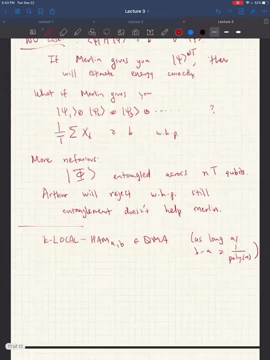 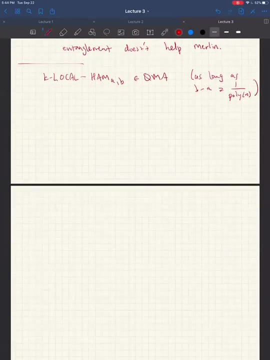 We've shown that local Hamiltonians are in QMA, which is the analog of NP, and now let's talk about QMA completeness. So what that tells us is this local Hamiltonians problem characterizes the complexity of QMA. Okay, and this brings us to the quantum analog of the Cooke-Levin theorem. 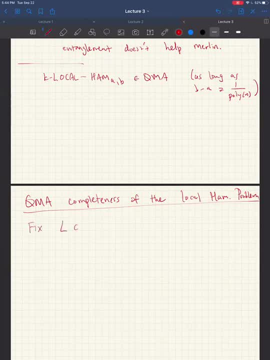 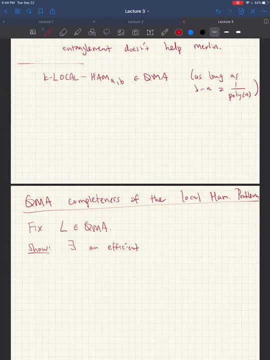 this is quite an efficient transformation of instances X for this decision problem into local Hamiltonians that are eight, nine, ten, 100, 100, barbecue barbecue, barbecue barbecue. instances of, well you know, such that if x was originally the s instance. 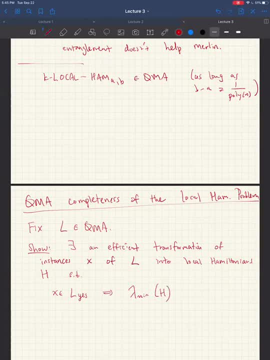 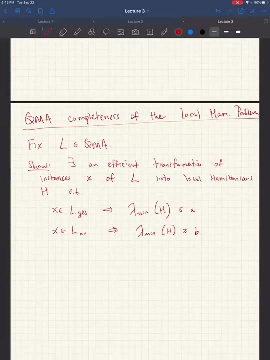 then the ground energy of h is going to be small, and if x is a no instance, then the ground energy is going to be high, as where low and high are characterized by a and b. So how do we do this? Well, we're going to try to follow the intuition of the 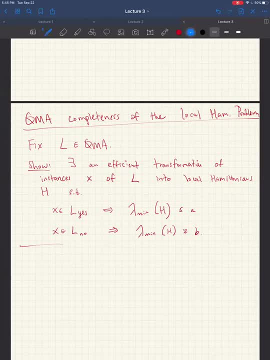 classical Cook-Levin theorem. So the fact that we have a QMA language here. well, let's just unpack what it is. Well, we have this family of verifier circuits, right, one for each input length, and so let's just fix an n for now. 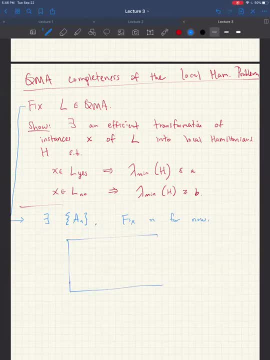 Okay, so we have this verifier circuit, this a sub n, and we plug in this x. Merlin will hand us a proof. We have some ancilla qubits, We do some polynomial length computation and then we can decide yes or no. instance with high probability. 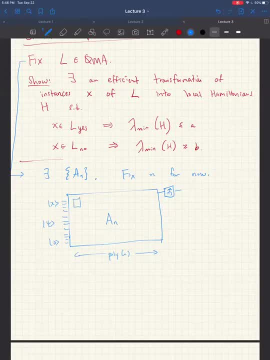 And, furthermore, let's just imagine, you know, what the gates inside the circuit might look like. This circuit consists of one and two qubit gates that are arranged in different ways, and let's call the gates u1,, u2,, u3, and so forth, All right up to the very last gate. So the ui's are one and two qubit gates. 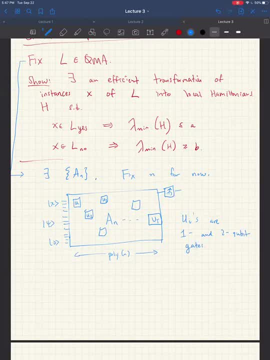 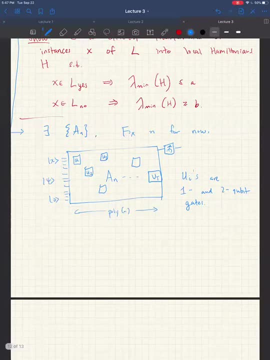 You know they're unitaries, Okay, so remember that. the Cook-Levin theorem. what was it doing? It was saying: you know you had some classical computation, this Turing machine, and you're going to like have a snapshot for every step of the. 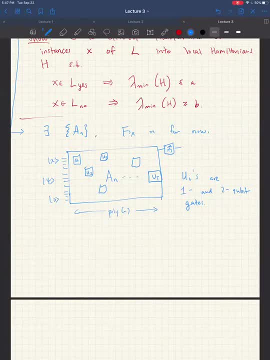 Turing machine. You're going to write each snapshot as a bunch of variables and you're going to have constraints on these variables to make sure that the snapshots really are valid, like they transition to each other in a valid way. Also, the snapshot, you know, the beginning snapshot starts okay. 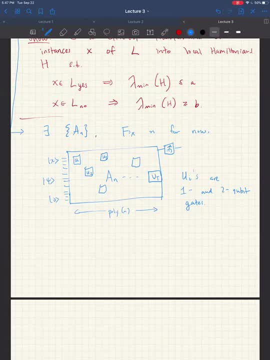 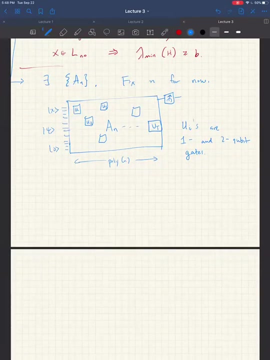 the ending snapshot ends okay and you sort of put all that together and you have a bunch of constraints that the only way to satisfy them is if the snapshots correspond to your verifier accepting on some proof. We're going to mimic that by creating this quantum constraint satisfaction problem. 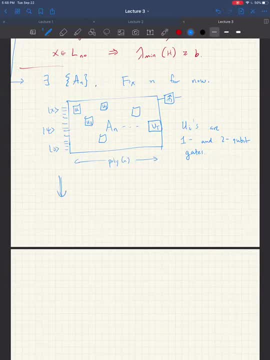 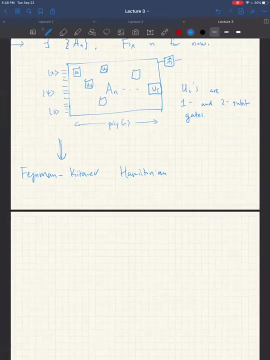 So this is: we're going to transform this into the Feynman-Kataev Hamiltonian, Which is named after Richard Feynman and Alexei Kataev, who kind of developed this idea. I'm going to call it H, and it's a bunch of terms. This H has ground states that look like this: 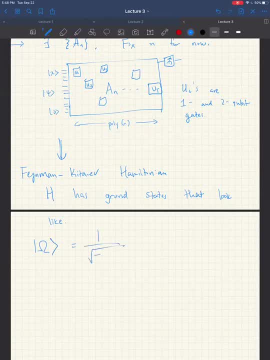 So I'm going to call it omega and let's say that our circuit runs for time t. It's going to be an equal superposition over all t plus one time steps of this circuit. We're going to have a register that keeps track of what time step we're interested. 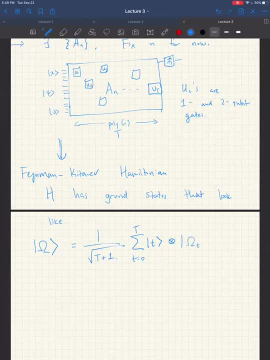 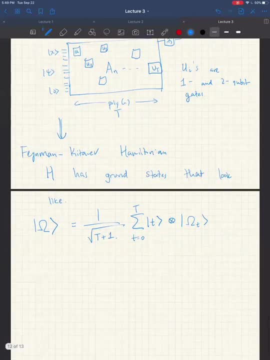 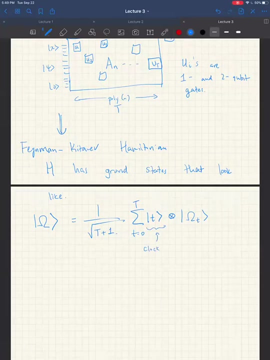 in and we're going to have a snapshot of that intermediate state of the computation. So this is what I call the clock. Okay, it keeps track of what time it is, and this is going to be the t-th snapshot of the computation. 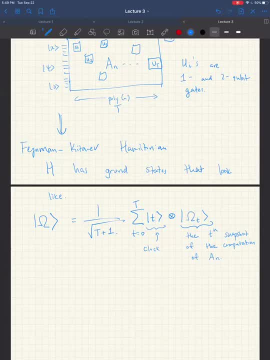 of a sub n. More specifically, for every intermediate time, t. this is going to be equal to some. you know all the gates: u t u minus u t minus one, u. one applied to the input of this circuit, which is going to be x, the supposed proof state, and zero. 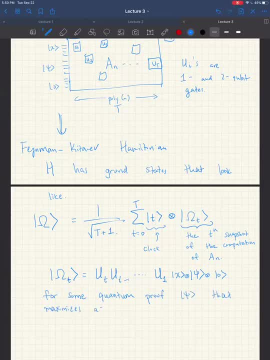 Then the uniform amount of the current number of times t? u and zero h equals one, is equal to the total and equal percent. So this is going to be the constant, the absolute number of times t? u. So we're going to design a local Hamiltonian that is going to have this as its ground state. 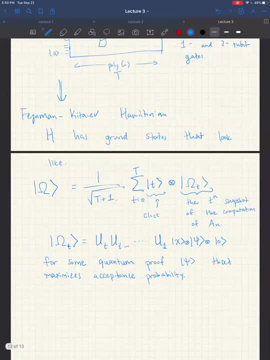 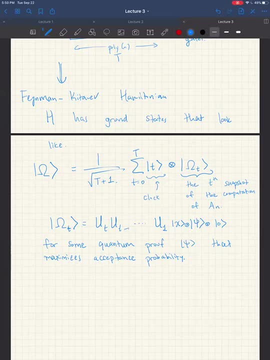 and it's going to be a very simple way of doing the actual longitudinally- lihat problems on this diagram. so if you're going to have, let's say, a random state, you can do this. So we're going to design a local Hamiltonian that has this as its ground state, and there's many 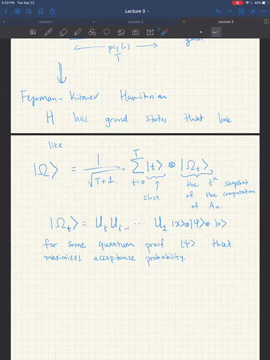 many choices of potentially many choices of ground states, because there could be many choices of quantum proofs that maximize the acceptance And we want to try this method, especially because there are other values in the model that maximize the acceptance probability. But whatever those states are the ground. 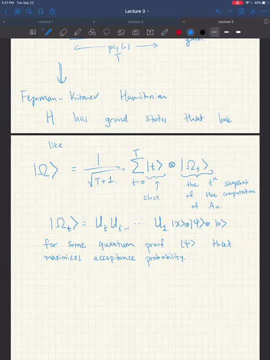 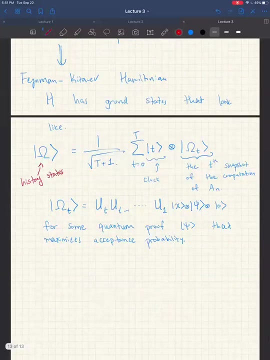 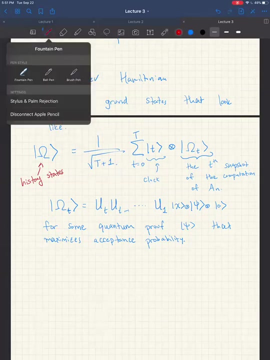 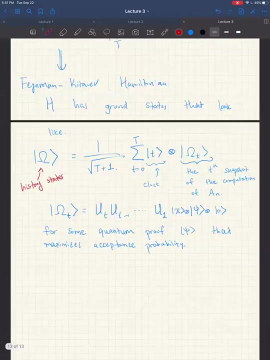 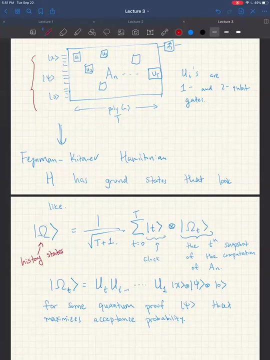 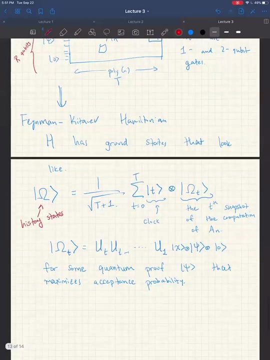 states must have this form, And these in particular are called history states because they tell the history of the computation of this verifier. And just to be clear, like you know, suppose that the number of qubits that this circuit acts on is I don't know. let's give it a number like r qubits, Then the history states. 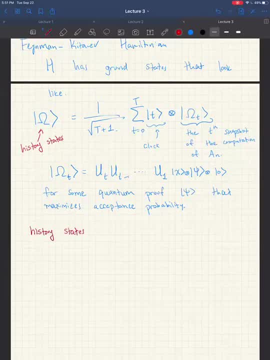 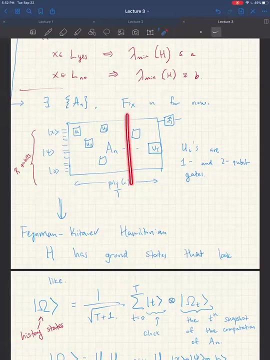 are on log t plus r qubits total. Why is that? Well, the snapshot part of it, this is r qubits, because you know the omega sub t will be like. if you just like, pause the computation at the t. 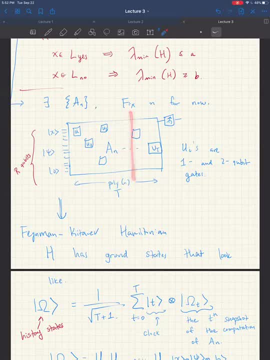 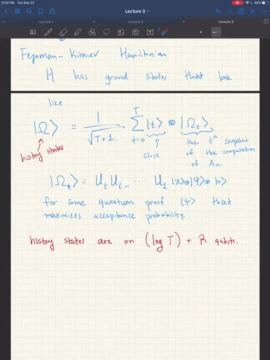 time step. that will be the quantum state of these r qubits And then this log t. here will be the number of qubits needed to represent what time it is. Since time runs through 1 through t, you need at least log t. 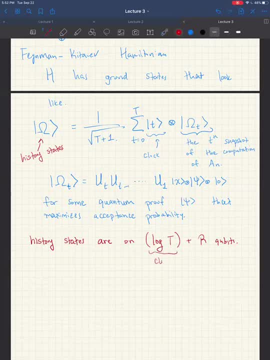 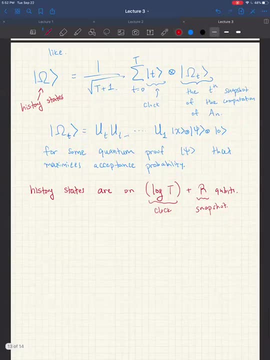 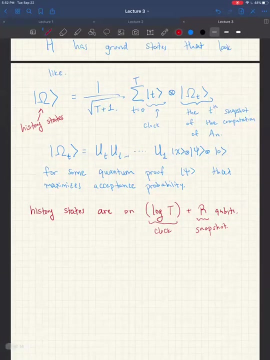 So this is for the clock and this is for the snapshot. Okay, So hopefully you can start to see some resemblance between, like, this history state and this Cook-Levin tableau that we talked about last time. Okay, Okay, Okay. 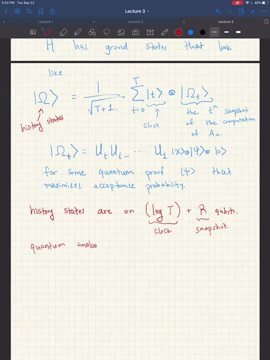 Okay, All right, All right, All right. The tableau had all these snapshots laid out on rows And you know you got it all at once. Here, the snapshots are laid in superposition. Okay, Okay, So that's the ground state we're aiming for. 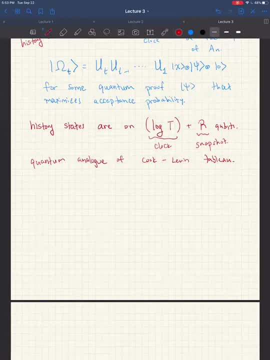 How do we但是ize this? do we design a Hamiltonian to obtain this as the ground state? Well, we're going to create terms that correspond to the starts okay, check, evolves okay and ends okay. The starts okay is to make sure, so we're going to have Hamiltonian terms. 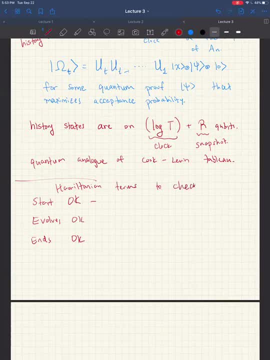 to check. We're going to check that this omega zero, the very first snapshot, which is the beginning of your verifier circuit, has this form And you want to make sure that the verifier algorithm starts with the right input, right The evolves. okay is to make sure that for each psi t it's equal to 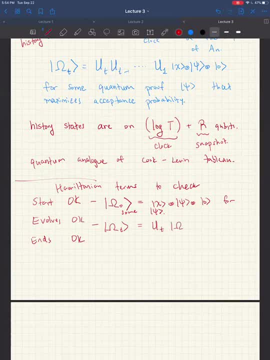 the t-th gate applied to the previous snapshot. And then the final check is to make sure that if you look at the very last snapshot measuring the output qubit of omega capital T, you'll see that the first snapshot yields one with high probability. 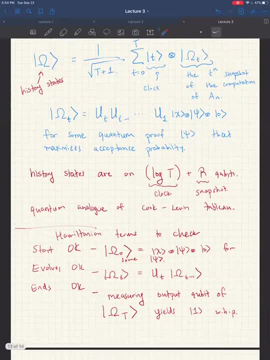 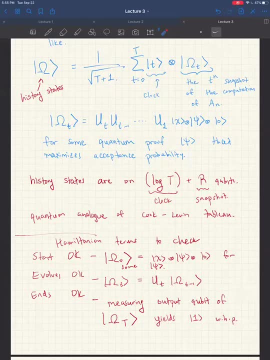 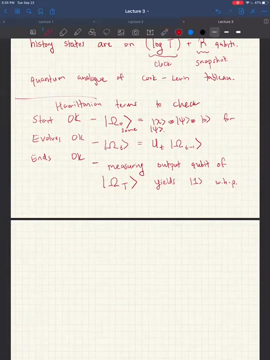 So if you walked up to me with some quantum state, some history state that satisfies, starts okay, evolves okay, ends okay, then what does this tell you? It tells you what the second snapshot yields and the third snapshot yields. It tells us how many data sets have been generated right here. 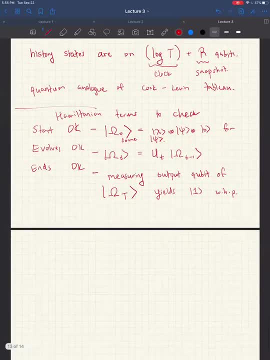 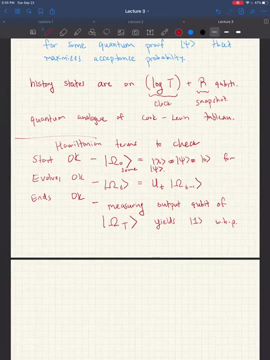 and how much data is still on the system, and now these data sets seem to be left behind. So let's make sure that the first snapshot yields the two output: qubit, rat And, as you can see, now, the current RDM is around 3.3 million. 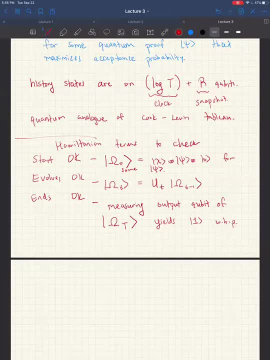 and then the second snapshot is around 3.5 million. Again, that means that the state will use the data set in the previous snapshot to determine the change in time. So the way that you can see is that you can see that the state is operating at the same time. 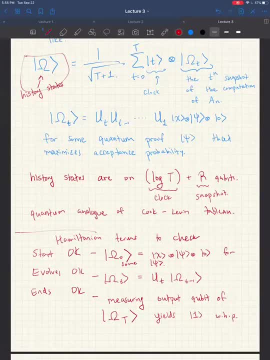 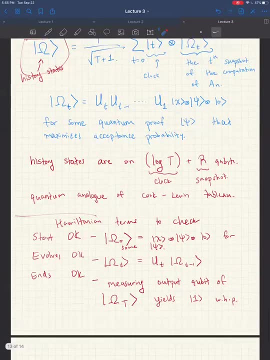 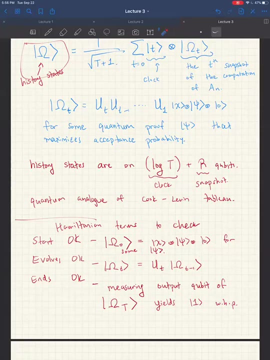 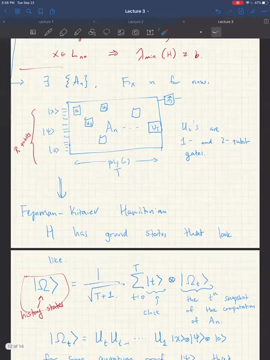 history state and you and you know that it satisfies each of these constraints, like: starts okay, evolves okay and it's okay what? what conclusion can you draw? this history state should be telling you a story, right like it should be proving to you some some fact about this original circuit. it's almost tautological. 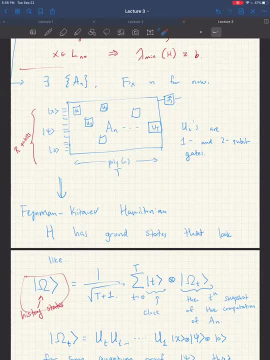 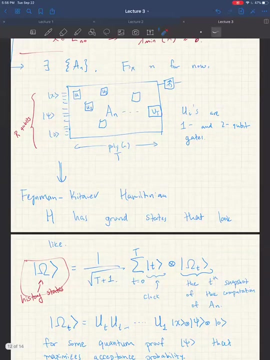 isn't just like: exists a circuit that solves the problem, So the circuit is fixed. Um, isn't it just saying that the- that circuit above does a valid computation which uh accepts with high probability? Um, like that- that problem in QMA, uh, or that algorithm is- is valid, Yeah. 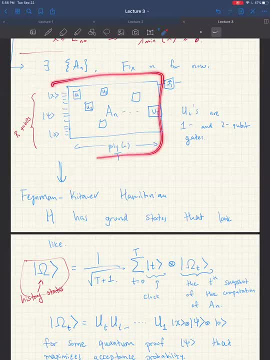 So- so we're fixing the circuit here and someone hands us a history state that tells us the circuit has- has- valid snapshots of this particular circuit at each step and at the end it outputs one with high probability. then you don't need to run the circuit yourself. 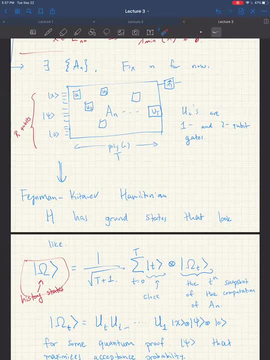 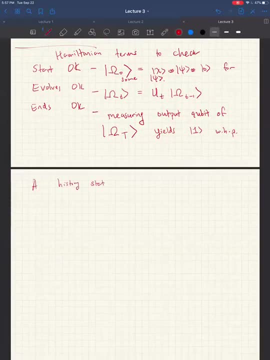 The-. the history state tells you that this is true. So how can we solve it? So it tells you that there is some psi. that's part of this history state. this circuit A on X sine zero outputs one with high probability. right, But what? 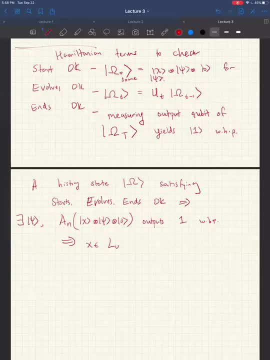 do we know about this verifier circuit? It tells us that that must mean X is a yes instance of your original language. Okay, so that's what this Hamiltonian is supposed to do, and I'll finish this up next time, but we're going to have a bunch of terms that corresponds to you. 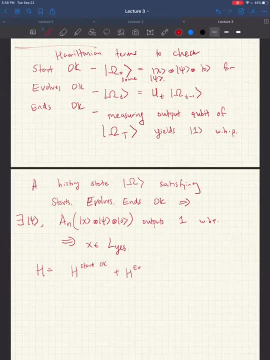 know, starts okay, evolves okay and ends okay, And actually each of these will work Okay. so that's what this Hamiltonian is supposed to do, And I'll finish this up next time, but we're going to have a bunch of terms. that corresponds to you. 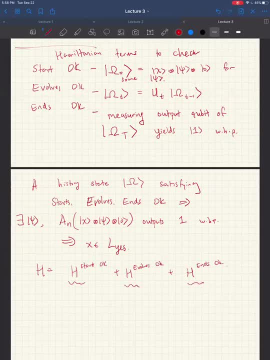 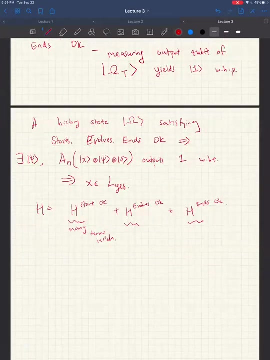 know starts okay, evolves okay and ends okay, And actually each of these will decompose into smaller terms, but it will be a local Hamiltonian and it really enforces all of these constraints. So it'll turn out that, whatever the acceptance, 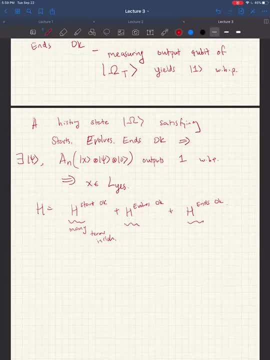 probability is like: yes, it's a yes instance of your original language. Yeah, so let's see. Well, okay, So the basic, the punchline, is that the ground energy of H will reflect whether X is a yes instance or a no instance. 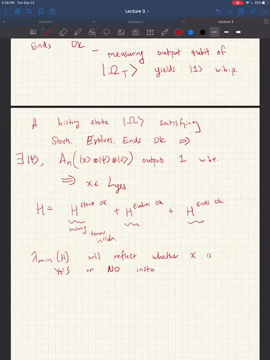 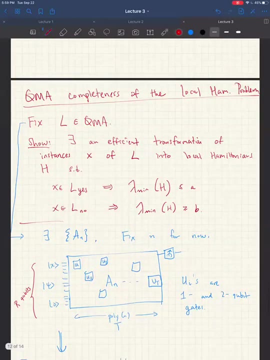 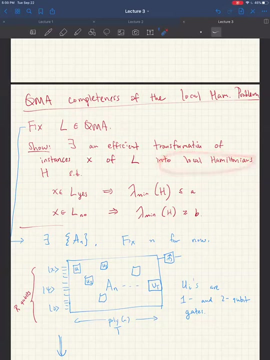 And that that completes this reduction And it shows us that we can encode arbitrary QMA problems as instances of the local Hamiltonians problem. Okay, So we're going to have a bunch of terms that corresponds to you know, ends okay and ends okay, And that that completes this reduction And it shows us that we can encode arbitrary QMA problems as instances of the local Hamiltonians problem. 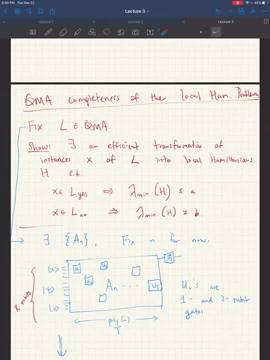 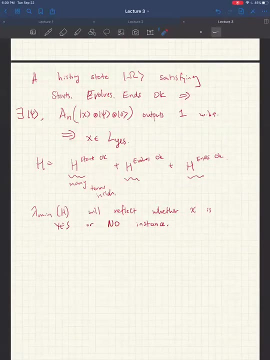 Okay, So that's it for today. I'm happy to stay out for a few more minutes and answer any questions that people might have. Next time I'll describe what this Hamiltonian looks like. We won't analyze every gory detail of it, We'll just talk about it at a high level. 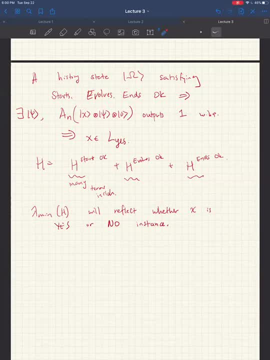 And then I'll jump into this thing called the quantum PCP conjecture, Which continues this theme of changing the notion of what we mean by a mathematical proof. Okay, so, thanks, Andrew. Andrew, you had a question right, So could I repeat what I said about the operator norm? Yeah, so the definition of the local Hamiltonians problem. we're assuming every term has. 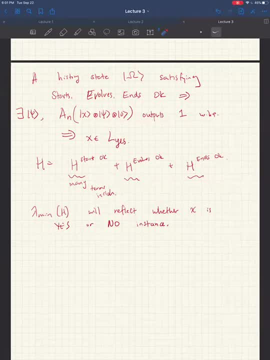 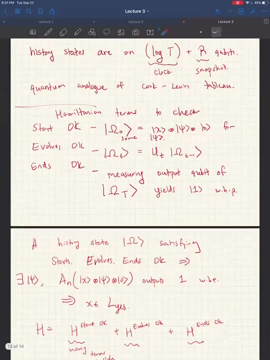 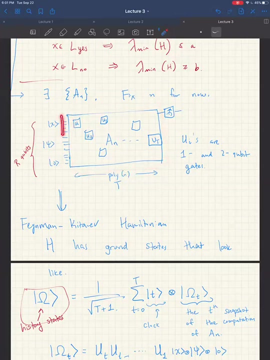 maximum i constant. What we mean by that is that every incubator source is just full polygon value 1. It's just to keep normalization consistent. Can you repeat what are was Our? is the number of keep its that? This Verifiers ticket X on. so are includes n. and then how many ever cupids you need for the witness and as many answer the qubits as you need. 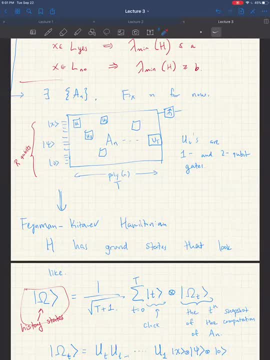 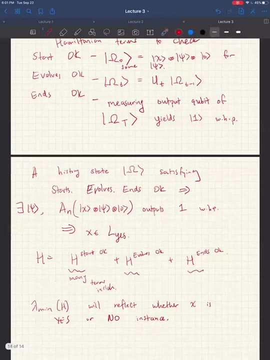 like k local Hamiltonian kind of becomes like a global kind of thing because it acts on all qubits now oh, uh, good, so I guess I haven't gotten there yet. um, these terms, uh, will actually be um. okay, the way of describing these terms will be um log t local. 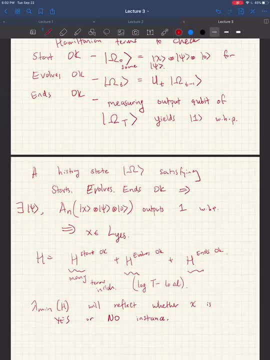 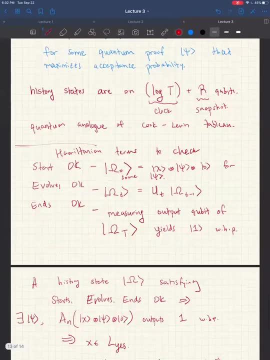 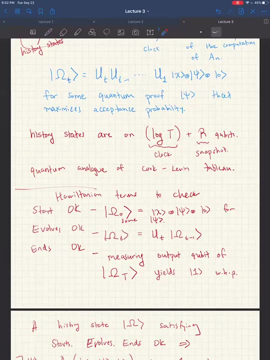 but it won't depend on r. okay, so those, those terms are different from the, the omega terms that we wrote before. oh, so the omega is just a state, right, so some, uh, there are no terms here, okay, okay, uh, can I ask a question regarding to the quantum circuits? 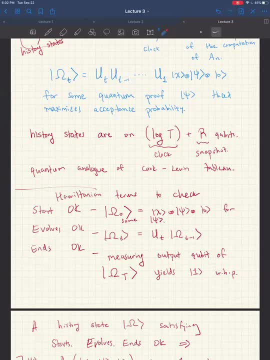 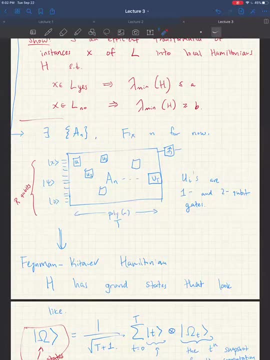 so? so imagine that the input to the circuit is classical. okay, classical states then, and every, every, every element in the circuit is, is k local, then can we simulate this quantum thing, quantum circuits, using classical circuit, because, because obviously we can use a finite lens of polynomial lengths of this to represent this. 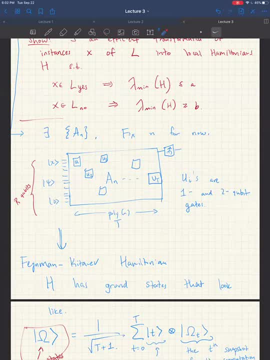 whole computation. right, if we have like infinite precision, you could don't care about finite precision, um. so, in general, no, because, even even if you allow yourself only two, two qubit gates, right, um, but the thing is these gates can introduce entanglement, so, uh, representing even after a 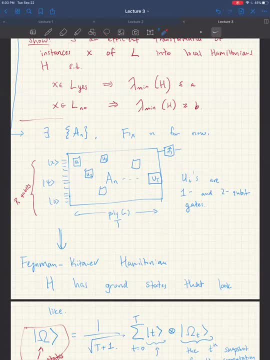 small number of these two qubit gates you can generate entanglement. that's so complicated that to write down the, the full vector of all, and n qubits in your computation, uh, would require um you need to keep track of like two to the n parameters. 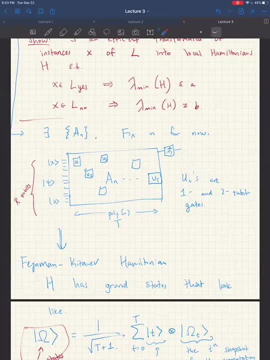 uh what? because it might, it might be that the explicit terms is two to the power one, but is it possible that we have something, uh, some measurement that is efficient, such that we can efficiently sample from this measurement, from this state, because we really, we really have a compact description for these states? 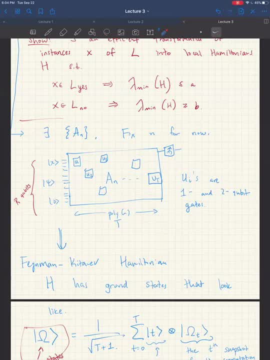 given this: uh, circuits right, oh, good question. um, so the whole belief is that it's not possible to, even though you're right, like, if you have like, say, a polynomial size circuit you can rep, you can describe the circuit efficiently, but then to sample from, say, the output distribution of the circuit. 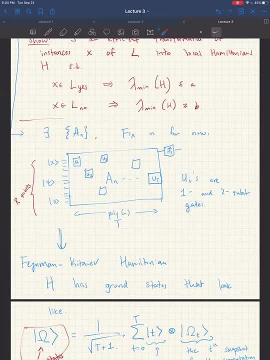 we believe is is actually intractable. we don't have a proof of this, um, but this is sort of the- at least the best complexity theory evidence is is that you cannot um and um. you know, i mean there's there's some like complexity theory proof in the. 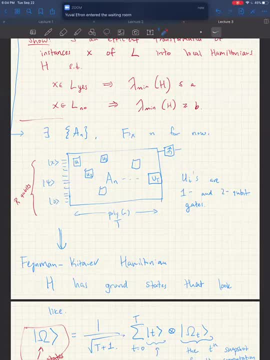 sense that if you could sample from this distribution exactly, then you could solve, uh, things that are provably hard, like you know, for example, computing the permanent of of some matrix. um, uh, you know so, so we know that's. um, uh, you know so, and you know, the assumption is that that's difficult. 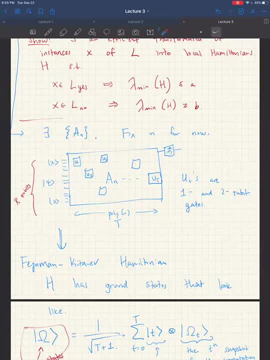 for, uh, um, for classical computers. yeah, in the, in the no case of the local hamiltonians. um, you were saying how if um merlin were to give us an entangled state, we would still reject the? um, we would still reject our, our ground state energy we would still reject because it's still be. 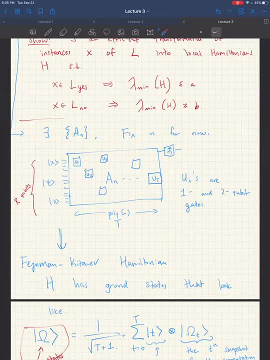 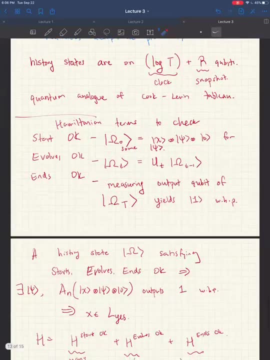 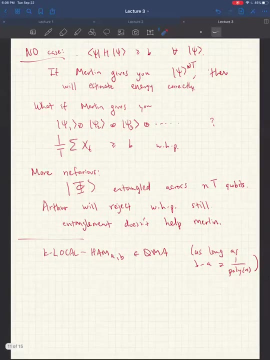 greater than b. that's not. could you just go through that again, because it wasn't really obvious to me? oh, it's not obvious at all. um, so i didn't, uh, explain the proof. it requires a proof. um, yeah, i, i may include this as a problem set, but, um, but, uh, the intuition is that i mean. 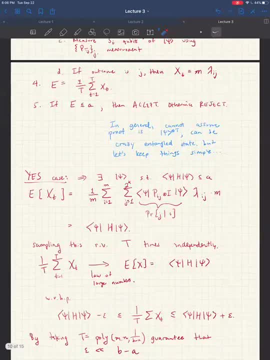 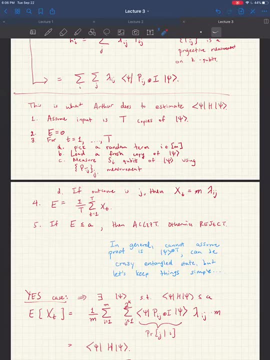 if you sort of look, analyze um, what um arthur is doing in this algorithm, he's, he's treating each of these uh registers independently, like each of these. i mean you divide them into blocks of n qubits, right, because you were thinking, you know, in our heads we're thinking each block is independent of each other. 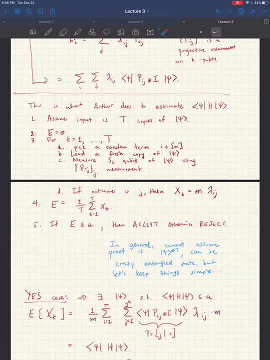 yeah, and so we're just going to measure one and and get an estimate, uh, and then, after we measure this, the first block of n qubits, this is going to, in general, collapse the rest of the state in some other way. and so we're just going to measure one and and get an estimate, uh, and then, after we, 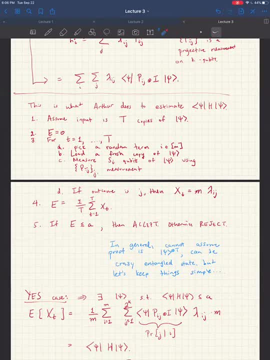 measure the rest of the state in some other way, because the whole state is entangled. but no matter how we collapse it, the next n qubits when you just consider them by themselves, cannot. uh the average measure. you know the average energy of the next n will still be greater than b. 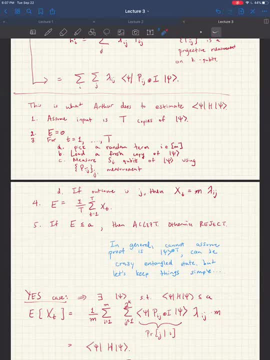 because there's no state that has energy less than b, and so then you perform the measurement and then that'll collapse, the you know, the remaining, and so on. you sort of can do the same thing, but you're not going to be able to do the same thing. 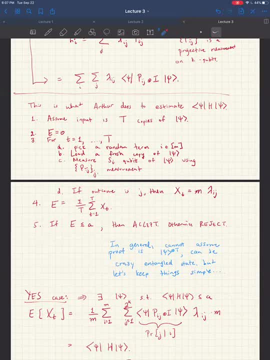 but you're not going to be able to do this iterative like uh measurement thing and you sort of argue that at all at all times. you know your estimates for these. the average of these, um, these random variables- x, uh, are always going to be at least b. 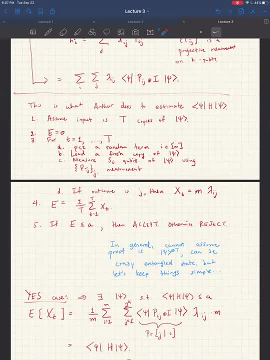 but it requires an argument. yeah, so it's. it's not obvious. so the quantum states are, are entanglements? looks pretty similar to a probabilistic drawn this distribution. so why do we really care about quantum computing? instead of this like, instead of like, uh, probably theory. 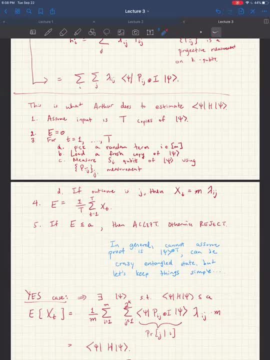 is it because of it's more realistic? uh, good question. yeah, it seems like it's similar to general probability, but the difference is in quantum. you can have cancellation, like you can essentially have what think of them as having negative probabilities which can cancel. you know, when you, when you sum up like a normal probability theory, when you sum things up, you can only add: 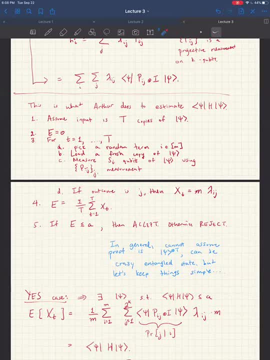 things like things never become less when you sum up probabilities. but with, uh, quantum information, you have these amplitudes which can be in general complex. so when you sum up a bunch of complex numbers together, these amplitudes, they can interfere and sometimes create a bigger number, or 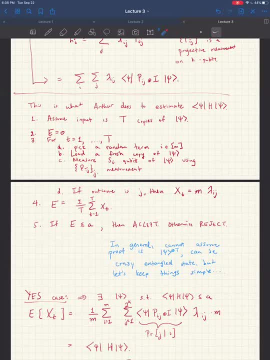 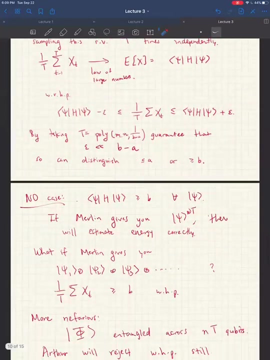 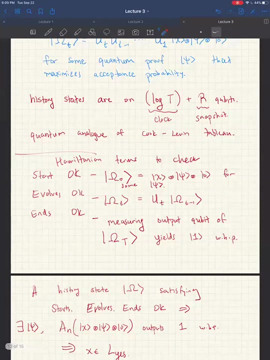 smaller number, uh, and that's gives a. you know leads to a big difference between classical probability theory and quantum information. i see that makes sense, thanks, yeah, um, maybe this was asked, but why is the locality of each of the terms of log t in this finding katai of hamiltonian? yes, at the end of the proof. yeah, um, it's not necessary um. 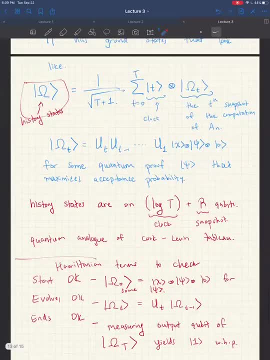 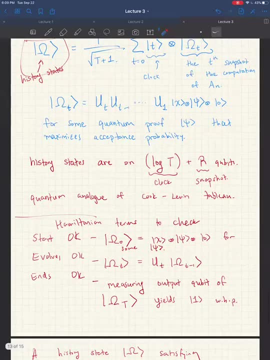 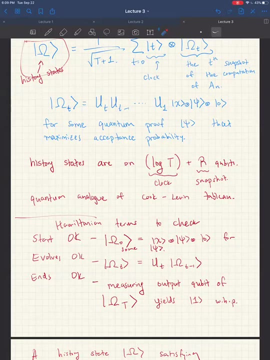 i mean, i didn't describe this actually, uh, because i didn't say what the terms were, um, it comes from, uh, i mean the way i'm representing the time stamp here, the clock. i'm representing the clock in binary. okay, so each of the clauses, you will look at the clock and 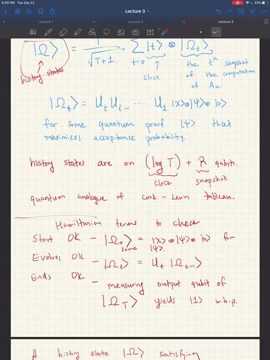 do something based on what the clock is. uh, there's a, there's a way that you can reduce the locality to a constant, say two or three, just by encoding the clock in a better way. basically, you encode the clock in unary. you just have, like you know, uh n ones to represent time stamp, uh n. 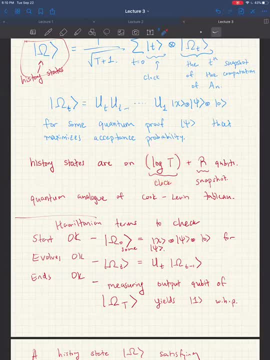 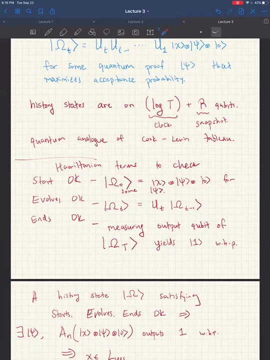 and there the locality will actually go down to like three or four, depending on your encoding. okay, thanks. so that means that even if i restrict k to be like three or four, the problem is still qma complete. yes, in fact we know that. uh, two local hamiltonians is qma complete. 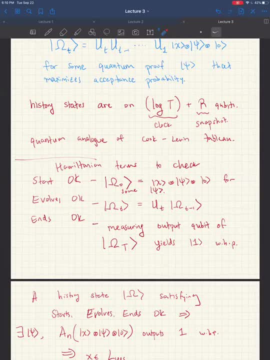 but there you need really, uh, exotic clock encodings. so the cię Garcia has, so there's the. so for the remaining people here, like, uh, i think, yeah, this would be helpful for me. are any comments about um sort of like the material so far? like it might go too fast, too slow? should we take more breaks? 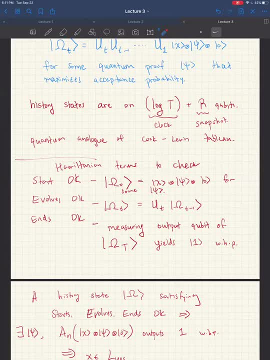 any feedback on that account. I think it's going at a decent pace. I don't know like. I look back at the notes occasionally, but I don't know. I feel like I'm following. Okay, good, Also very interesting stuff. 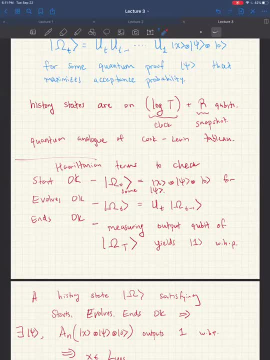 Yeah, it's a cool mix of things. It looks interesting, but I really I don't have a sense that I have an intuition, Like I'm catching glimpses of what you're saying. So I'm wondering if there is. I mean, I guess I can go through the lecture notes again, but 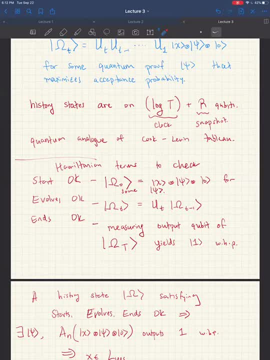 is there like a text that can give a bit more of introductory sort of material to this? I presume most of your students in this course have a some sort of quantum or mathematical background. for those of us who are from engineering, who are encountering this for the first time, you 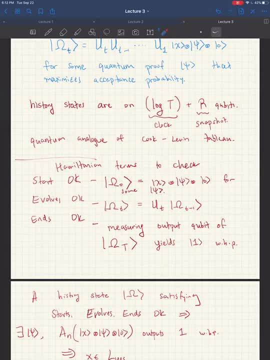 know like, do you have some recommendations for that? Yeah, I can provide recommendations, you know. unfortunately there are no. you know, this stuff is pretty new so there's not like any definitive textbook. I can send you different lecture notes on that. people have covered. So what's your background?